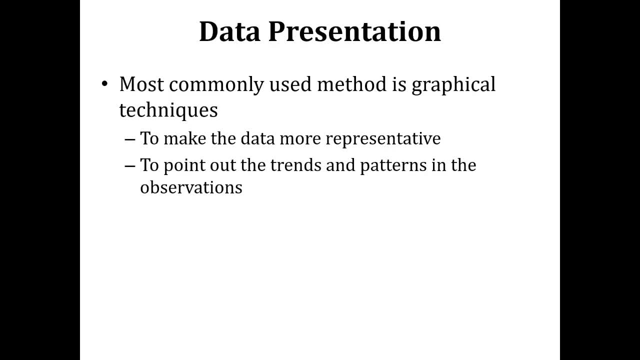 So the graphical techniques: they always make data more representative and they make data more meaningful to understand. So graphical techniques, or making graphs or charts, it is the most commonly used method of data presentation in science And there are different types of the graphs that you can use. but that depends on the type of the data that you have. 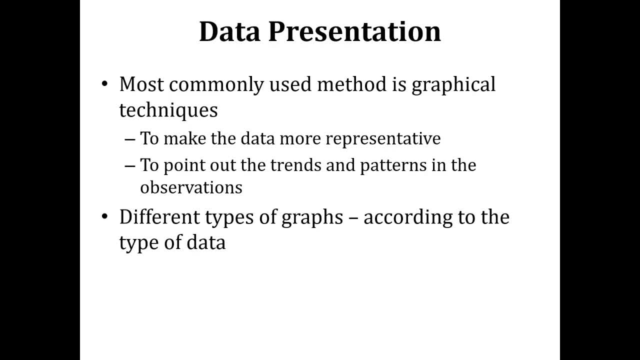 So it is not that every kind of a graph is suitable for any kind of a data. No, There are different types of the graphs that are suited only in some specific types of the data, for some specific types of the variables. So, looking at your data, you have to choose that: what type of graph you are going to. 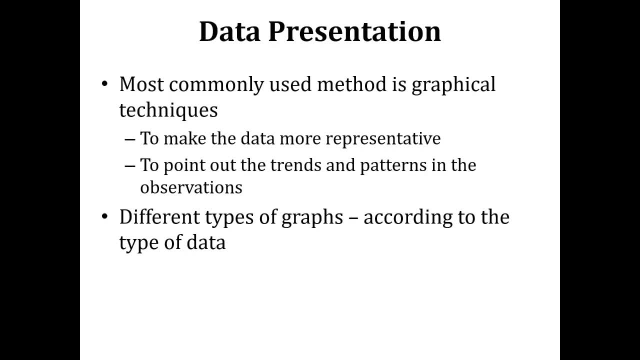 use. So the choice of the graph is again the fundamental concept or it is the fundamental decision that you have to make. So the fundamental concept or it is the fundamental decision that you have to make in presenting your data And all of your data presentation, it depends on the choice of the graph. 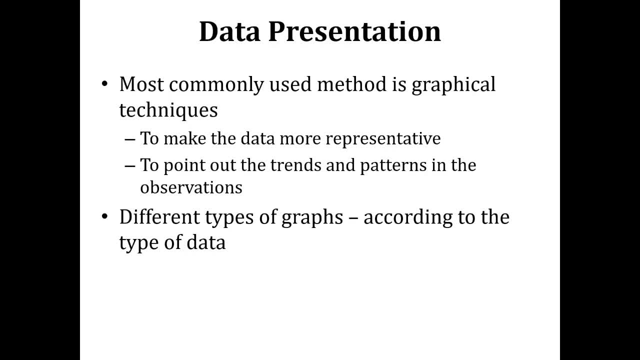 the choice of the graphical technique, the choice of the chart that you are going to use to present your data. So this is particularly important, that you are going to choose the graph according to the type of your data, according to the type of your observations. 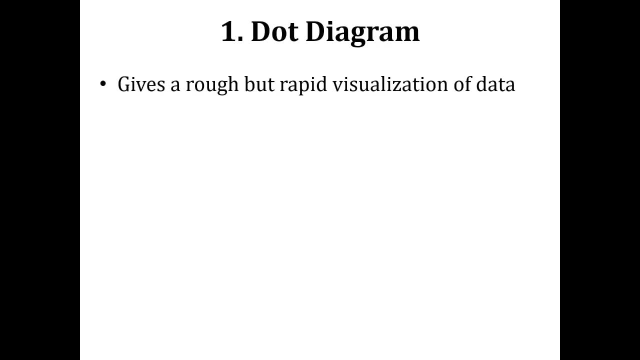 Now we are going to discuss some very basic types of the graphs and we are starting from the dot diagram. Dot diagram: it gives a rough but rapid visualization of data and it consists of a horizontal line which is marked out with divisions on the scale. So here you can see that we have a 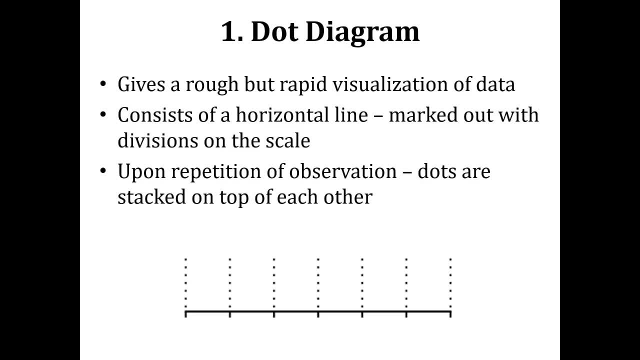 horizontal line, which is the solid line here, and then you can see that it has been marked on a scale. So there it so. this line is divided into different units and it is according to a scale. And you're just going to put a dot in place of your observation. So, upon repetition of the observations, dot. 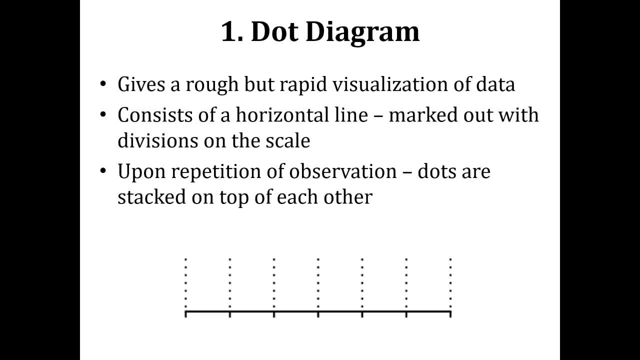 dots are stacked on top of each other. So this is the most basic type of the graph. but this type of the graph is only for the rough visualization of your data, especially when you are in field research and you don't have access to your computer and you want to just see that. 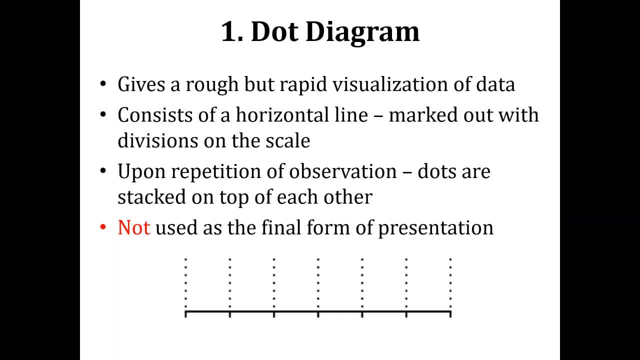 what are the trends in your data? what are the trends in your observations? So you're just going to make a dot diagram and this dot diagram is not used as the final form of presentation. So this is more of your rough work that you're going to use during taking your observations, or 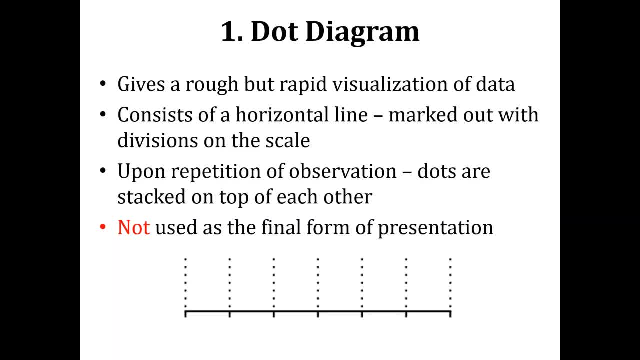 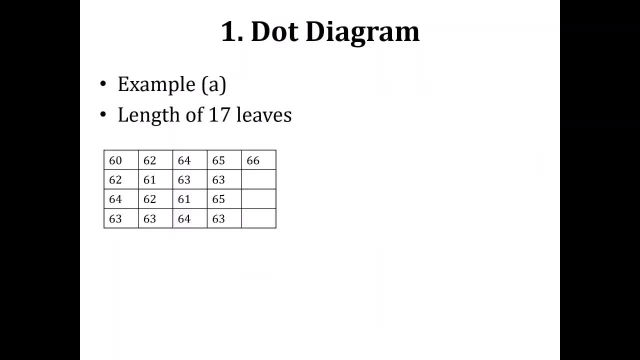 deducing some initial results out of your observations, So this is not used as the final form of presentation. Now we are going to see that, how we can use the dot diagram to see the trends in our data, to see the initial trends or patterns in our data. So we are taking 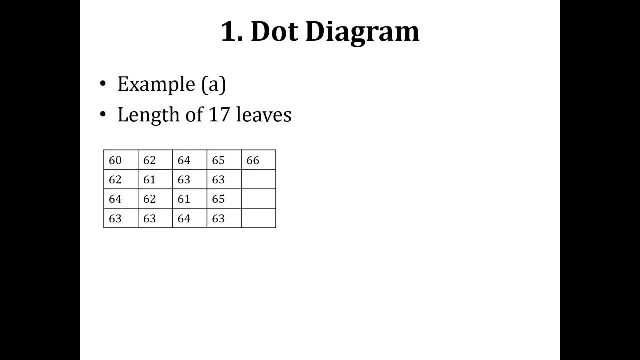 the example of the length of leaves, and we have 17 observations here and let's start making the dot diagram for this data. So here we have the horizontal line and it has been marked with the scale and you can see that this line is divided into a scale and the scale starts from the lowest. 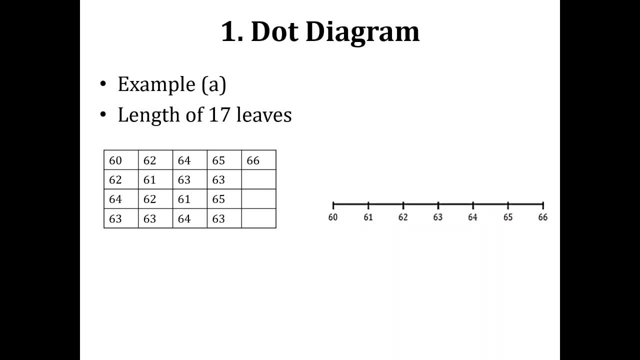 and it goes up to 66, which is the highest observation in our data. So this has been divided one unit apart. Now, when we look at the data, our first observation is 60, right? So what we are going to do is we are going to place a dot over 60, right? So we are. 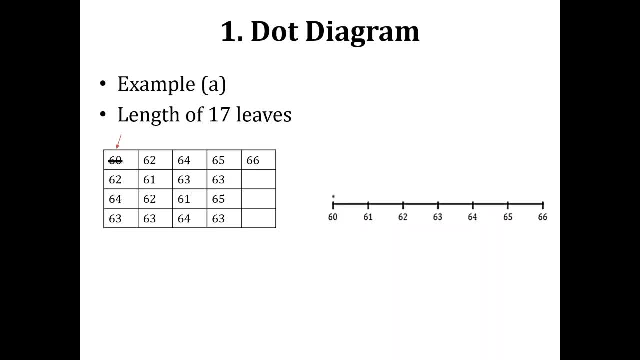 going to place a dot over here and we are going to mark out that this observation has been plotted. And then the next observation is 62 and we are going to put a dot in front of 62 on our dot diagram and we are going to mark this one. Then the next one is 64 and we are going to put a dot. 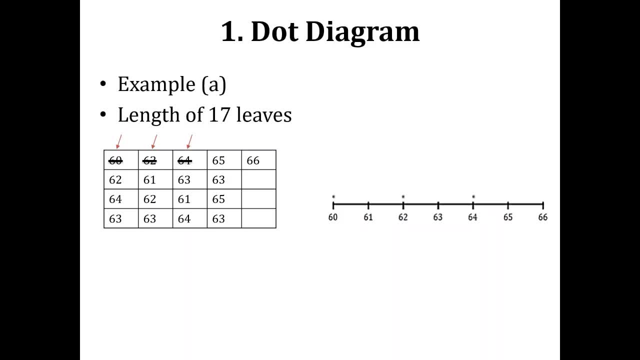 over here in front of 64 and we are going to mark this out, And then the next one is 65. So we are going to place a dot over 65 and we are going to mark it here. And then the next one is 66 and we are going to place the dot. 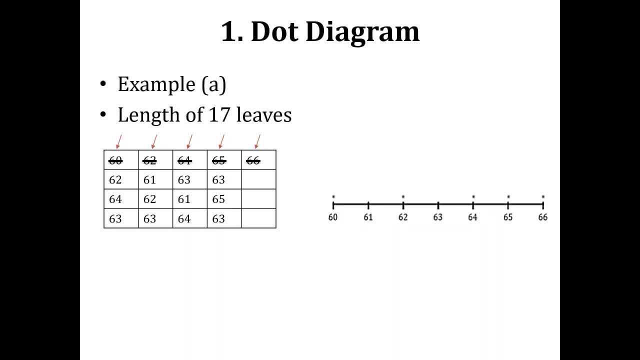 against 66. We are going to mark this out. Then the next observation is 62. So let's see. So there is already a dot in front of 62. So we are. what we are going to do is we are going to stack the next. 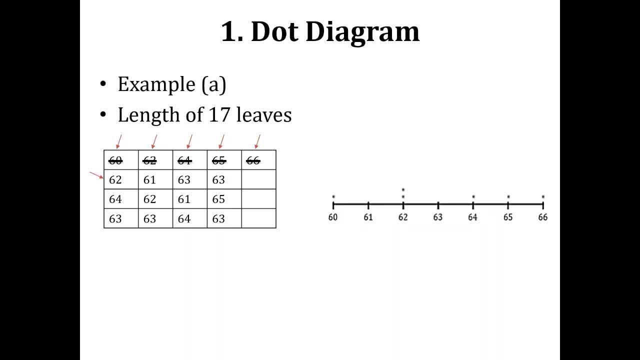 dot over this one. So here is the second dot. So this is how we are going to place the dots in front of all the observations that we can see from our data, And we are going to get our final graph here. So here you have, placed all the observations in the form of dots onto the diagram. 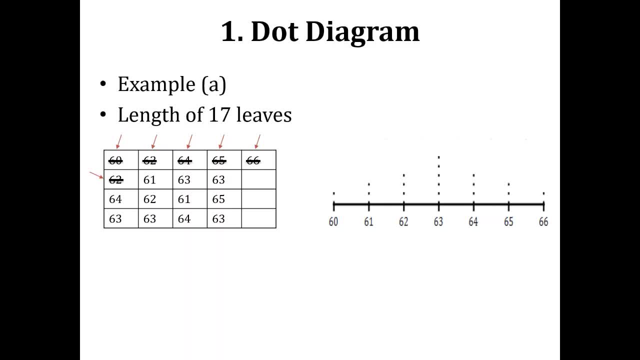 So this is the dot diagram that you have. So what you can deduce from this dot diagram? is there anything visible for the trends? Right, So you can see that your observations are scattered over 63 millimeters. Right, So you can see the trends in this dot diagram. quite. 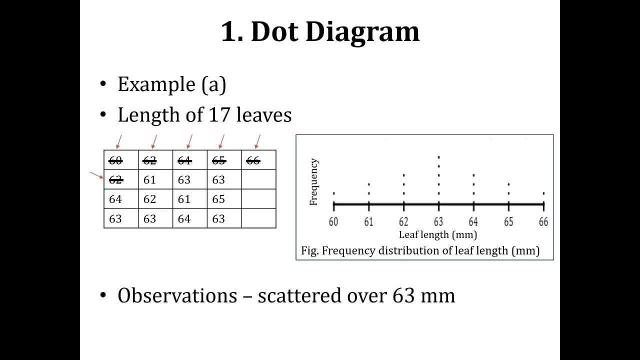 easily. And again because this is a figure, so you have to describe what this figure is about, Although this dot diagram is not the final form of your presentation, but still you are going to use it in your rough work, So therefore you have to properly label this. 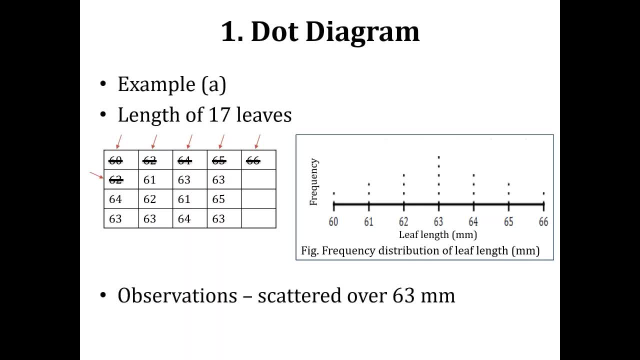 diagram And on the horizontal axis which you have, you have the leaf length, which is presented in millimeters, which has been measured in millimeters, And it starts from 60 and it goes up to 66.. So the horizontal scale, or the horizontal axis, or the X axis of this graph, 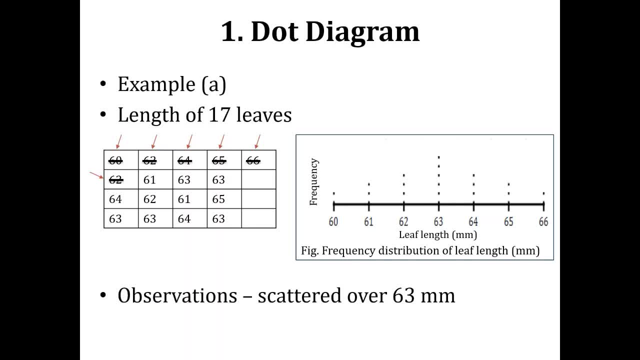 shows the leaf length. And what is the Y axis about? Y axis is about frequency. So here we can see that the observation number 60 on the X axis has a frequency of one, which means it is presented in the data only once, And then the 61 has a frequency of two. It means that in our 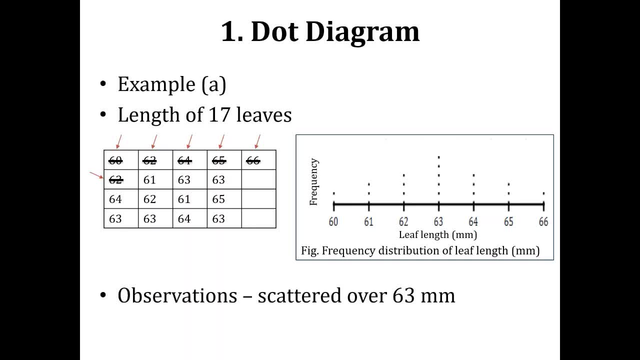 observations. we have two observations which are 61,, which measure to 61. Then is 62. And we can see that there are three observations which are measured as 62 in our whole data. Then we can see 63. And in 63, how many dots do we have? We have five dots. It means its frequency is five. 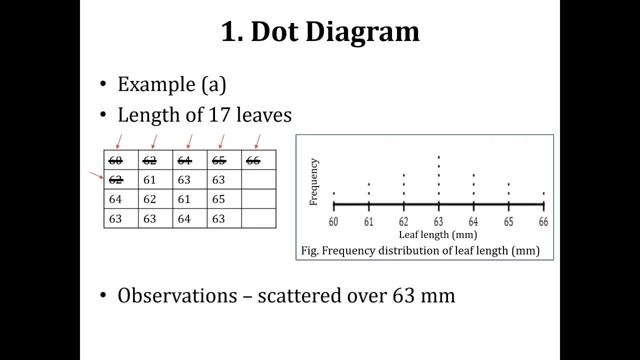 And then the 64, it has a frequency of three, 65 has a frequency of two And 66 has a frequency of one. So it gives us a quick visualization of our data. with what are the trends in our data And we can see that our observations are scattered over 63 millimeters. So this is how you make a dot. 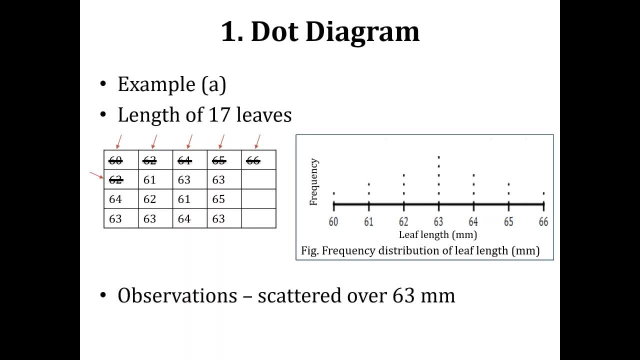 diagram for the rough visualization of your data And you have to give the caption as well. this figure represents the frequency distribution of leaf length. So in the figure you're going to describe the variable which has been plotted in this graph And also you're going to define. 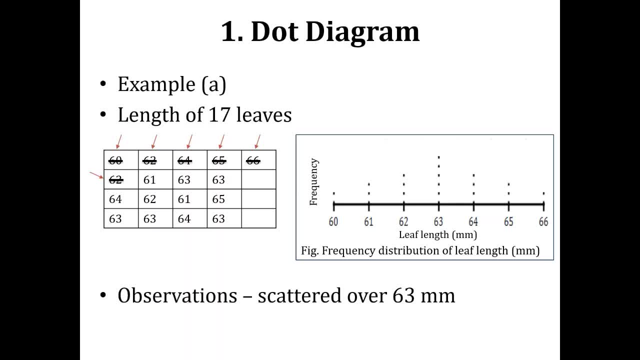 that what attribute of the variable is being described here. So you're describing the variable which is leaf length, And how you're going to describe this variable. you're going to give the frequency that how many times a specific measurement, a specific observation is repeated in your data. So this is how you make the dot. 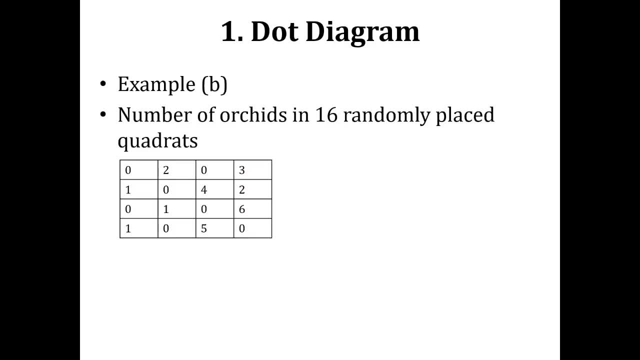 diagram. Now we are going to take another example for the dot diagram And this is about the number of orchids in 16 randomly placed quadrants. So in the previous example we took an example of a variable which was measured on the measurement scale, And now we are going to take the observation. 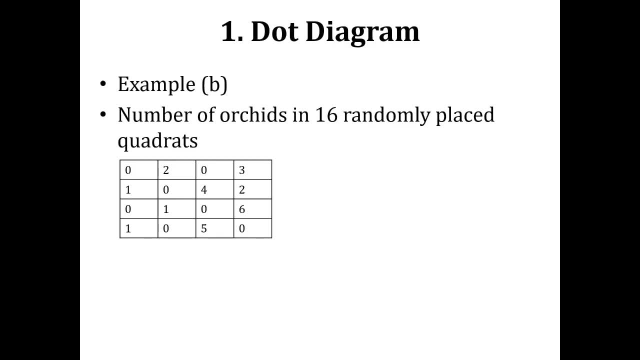 of a count variable, which is actually the frequency. So we're going to apply the measurement to our data, the count of things. So in this case we have the number of orchids, and the number of orchids have been counted from 16 randomly placed quadrants, and these are the observations of those 16. 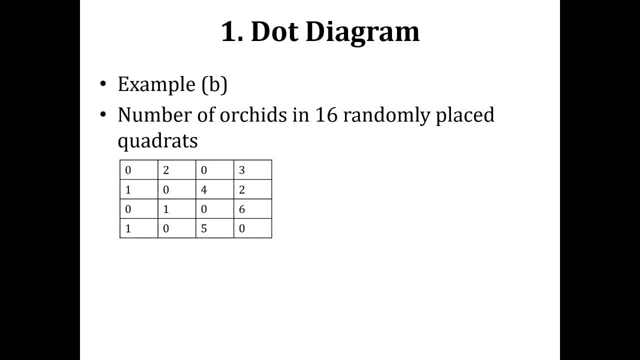 quadrants. So zero represents no orchid count in that quadrant, two represents two orchids in that quadrant, and so on. So this is our data and let's see how we are going to make the dot diagram for this data. So here we have the dot diagram and again, starting from the lowest observation, we 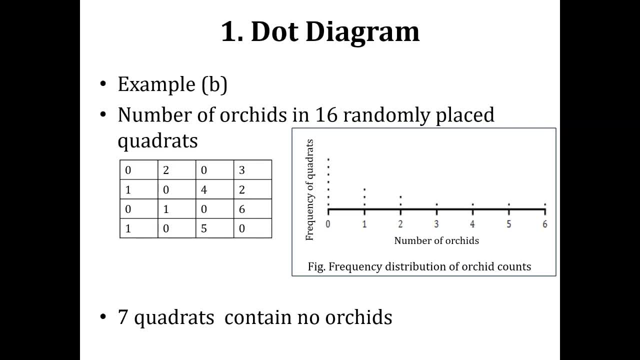 have zero and going up to the highest observation, which is six. So you can see clearly from this data that there are seven quadrants that contain no orchids. So you get a quick result out of your data and you can easily see that, what this data is about and what trends are visible in this data. 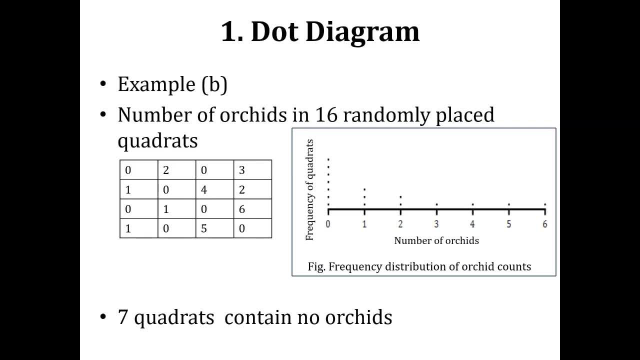 So in this case also, you have to properly label the dot diagram and you can see that we have given the caption, which is frequency: distribution of orchid counts. So in this case the variable is the number of orchids and what we are plotting on the y-axis is their frequency. right Now we discuss. 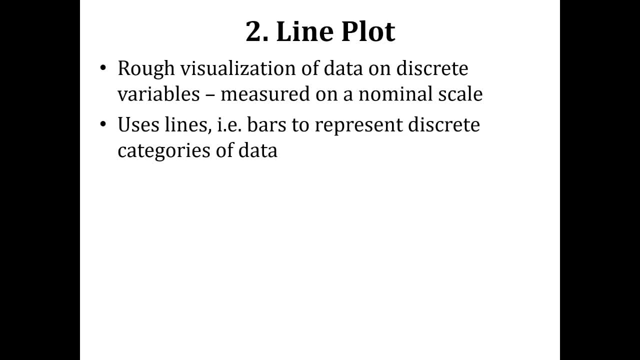 another type of the graph, which is the line plot, And again, line plot is used for the rough visualization of your data on discrete variables which are measured by the number of orchids. So this kind of the graph is usually used for representation of the count data and this is used 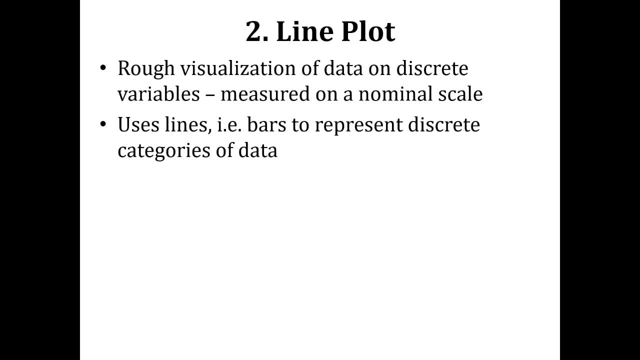 for the description of the discrete variables which are measured on a nominal scale, And it uses lines, which is, that is, bars, to represent discrete categories of data. Example is: you have 31 nest boxes placed in a wood and they're occupied by different bird species. So we can see: 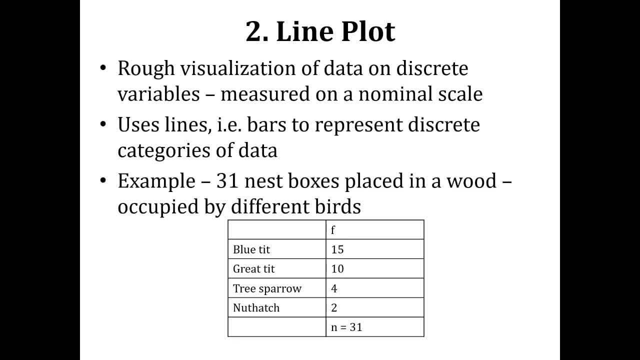 that there are 31 nest boxes placed in a wood and they're occupied by different bird species. So we can see that there are four bird species and they have occupied these nest boxes. So how many boxes do we have? We have a total of 31 nest boxes right And we can see that they have been occupied. 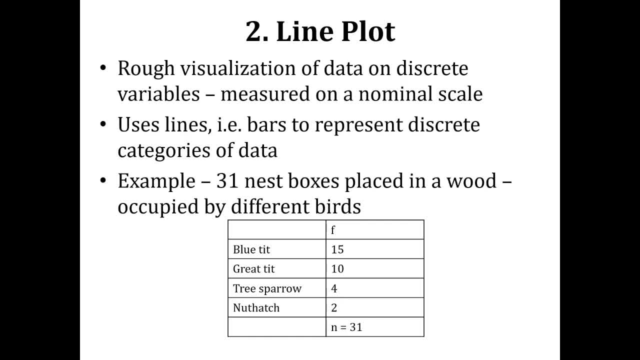 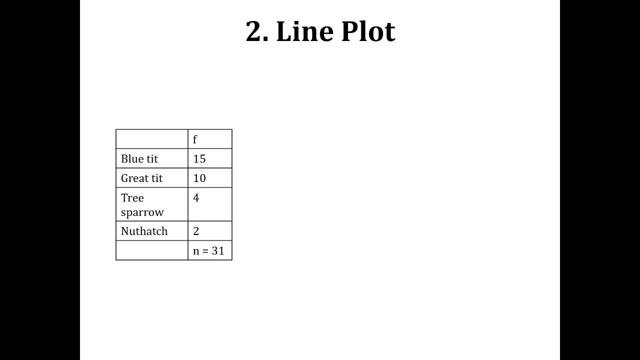 by different species of birds. Now we want to make a figure or we want to make a plot of this diagram, of this data. So we have our observations here, in which we have counted the frequencies, and we are going to make this plot, And in this plot, again, you can see that we have labeled. 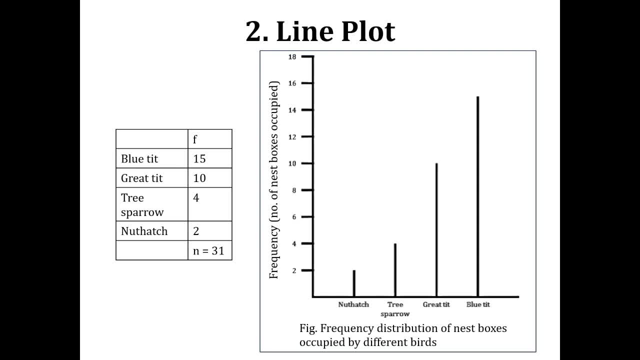 everything properly. The figure is frequency distribution of nest boxes occupied by different birds, And in this caption you can see that we have defined which is drawn on the x-axis and which thing is drawn on the y-axis. right, So we have defined everything. 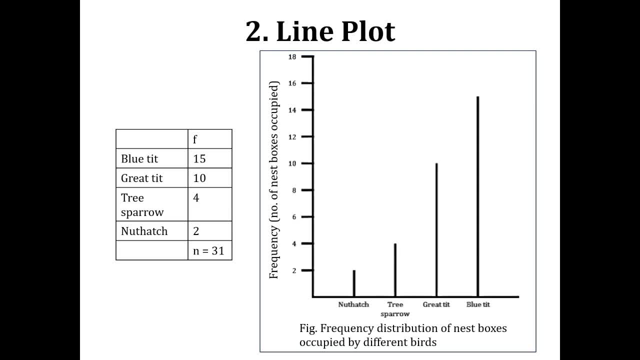 Then on the, we have also defined the axis, We have also labeled the axis. So on the x-axis, you can see that we have the names of the species, because these are the nominal categories. So we have names of different categories, We have names of different classes And these are the names of 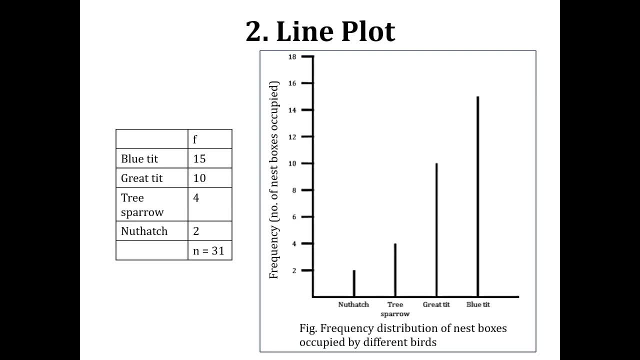 different birds, And then on the y-axis, we have the frequency and which is the number of nest boxes which have been occupied by a specific species. So we can see that the highest number of boxes have been occupied by the blue chit. 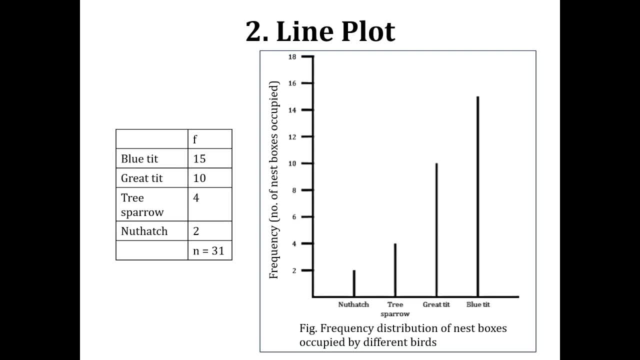 And the least number of boxes, which is two, has been occupied by nuthatch. So here we can have a rough visualization of our data. And again, this line plot is about the representation of nominal categories over a scale right. So this is how we make the line plot, And line plot is also 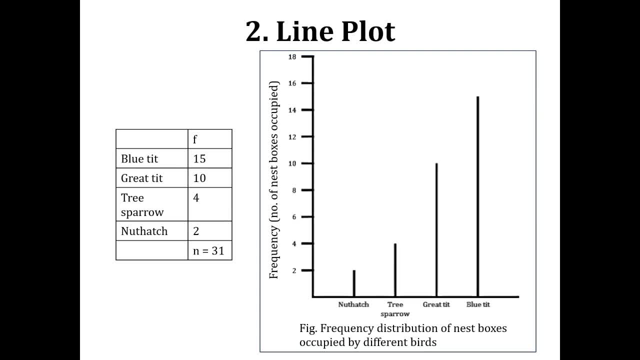 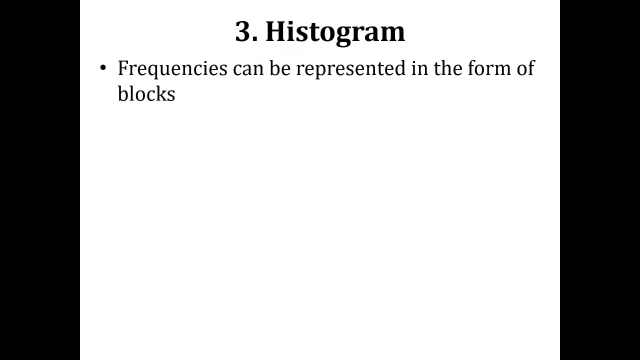 not a formal or the final form of presentation, So this is just for your own visualization, If you want to quickly look at what are the trends in your data, what are the trends in your observations right Now, after defining the two basic types of the graphs that you can use for 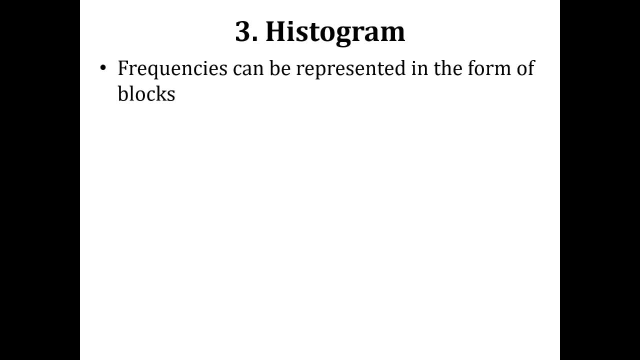 your own work, for your own visualization of the data. now we come to the most commonly used type of the graph that is used in the presentation of scientific observations and for the presentation of your data in your thesis, in your papers and in your presentations. So- histograms. they are the most commonly used type of the graph. 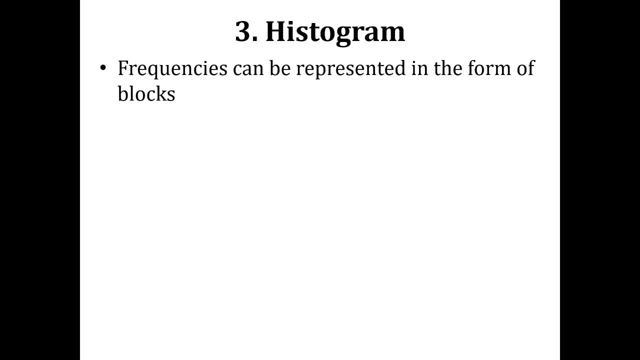 in scientific research. So in histograms we can represent frequencies in the form of blocks And the histograms. they are particularly useful for continuous variables, but they are used for the count data as well, And we are going to take the example of count data. 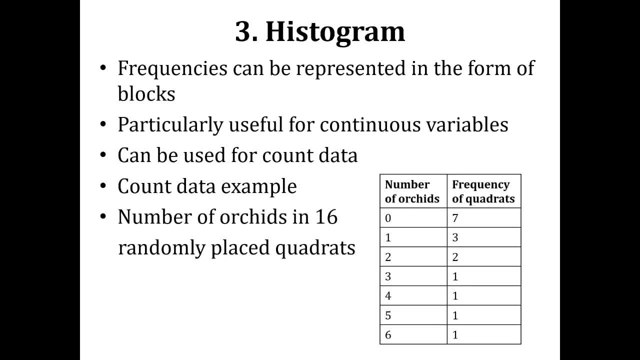 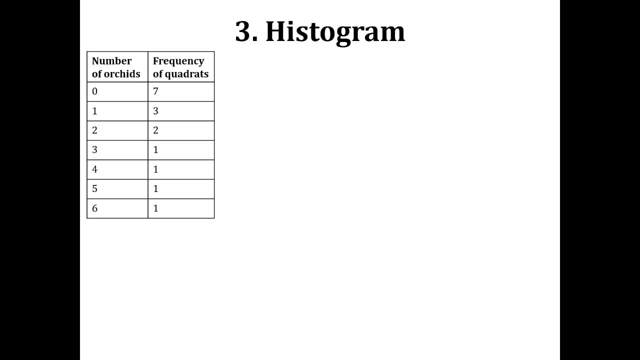 first. So here we have the number of arcades in 16 randomly placed squares. So we have the number of arcades and the frequency of quadrants, And now we are going to make the histogram for this type of the data, And here we have our observations, and which are the number of arcades and the frequency of the. 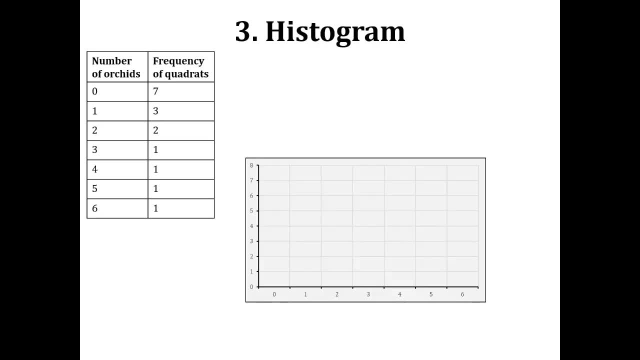 quadrants. Let's start by making the histogram, And here we have the histogram, the chart for the histogram, And in this one you can see that we have the x-axis and the y-axis. So what is there on the x-axis? The x-axis represents the number of arcades and the y-axis 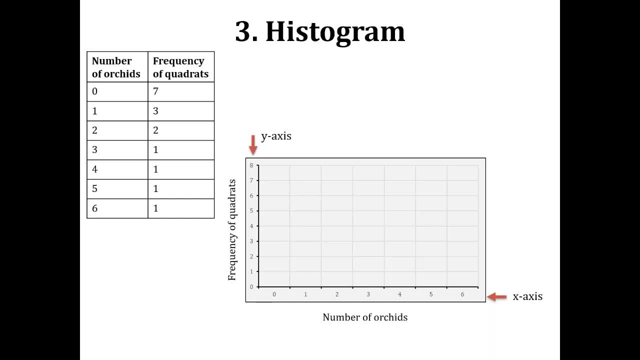 represents the frequency of quadrants And we have drawn scale over these axes as well, So the number of arcades, because they start from zero and go up to six. so we have scaled from zero to six on the x-axis, Then on the y-axis, our frequencies, the highest frequency is seven and the lowest frequency. 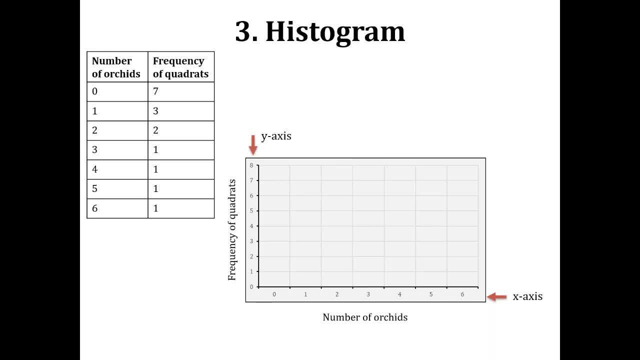 is one. And then on the y-axis, our frequencies: the highest frequency is seven and the lowest frequency is one. So we have started from zero and we have taken up the scale up to eight. So the making of the scales, it is up to you that, from where you want to start your histogram. So in this data we are: 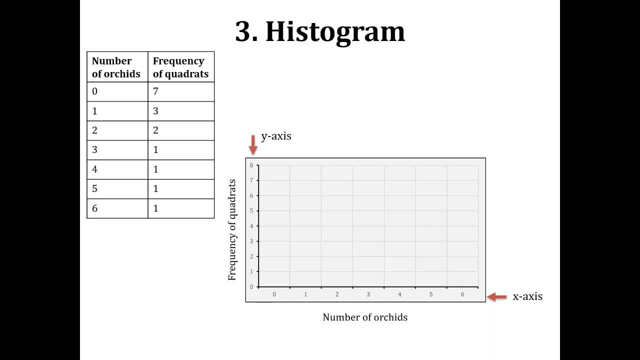 starting our histogram from zero on both axes and we are taking up the observations, up to six on the x-axis and up to eight on the y-axis. So this is the basic structure of the chart that we are going to make our histogram, And then you can see that we have the x-axis grid lines and we have the y-axis. 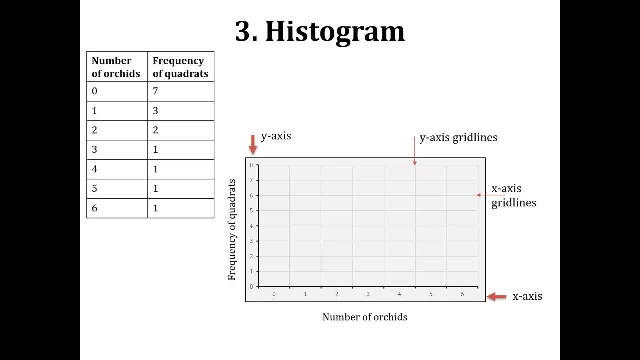 grid lines. Now, what are these grid lines for? So these grid lines are to help you locate your observation onto the chart to draw it. So the grid lines, they are basically going to help you when you're going to make your graphs manually on the paper, right? So these grid lines, they're. 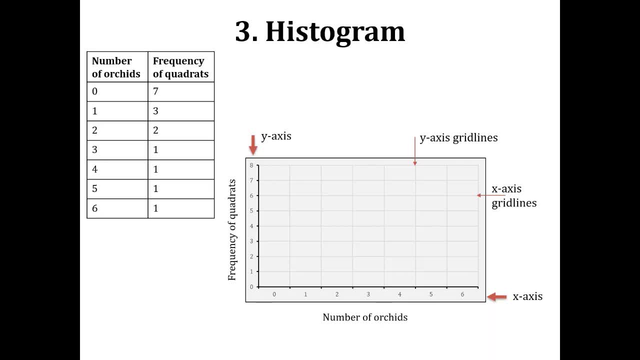 really helpful in making the graphs on paper because in that way you are going to easily scale out your observations onto the chart. that where on the chart your values should be placed. So this is kind of a scale that you have to draw your histogram. 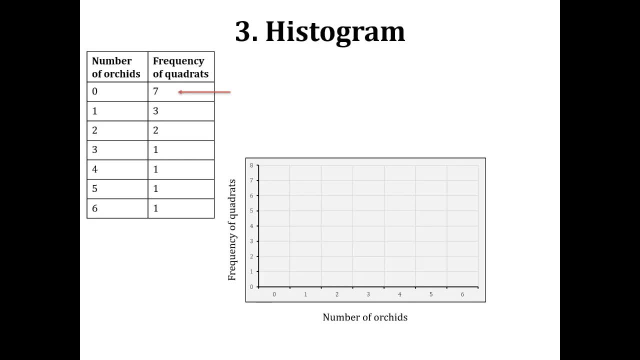 Now let's start by making the histogram. So here we have the first observation, which is zero number of arcades and the frequency of quadrates is seven. So on our chart it has to be here, right? So zero is the value of the x-axis and seven is the value of the y-axis. 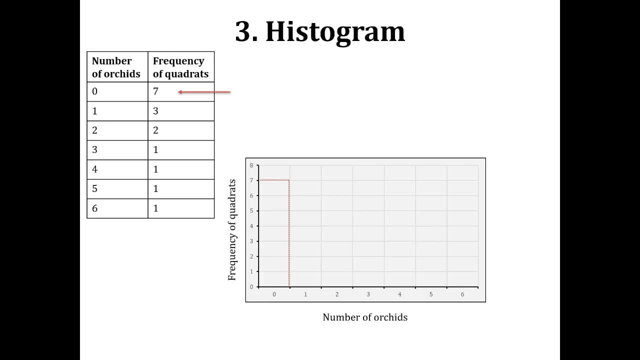 which is the number of quadrates that have zero arcades in them. So this is our block and we are going to make a block in this one. So we have our first block on the histogram and this block corresponds to the number of arcades zero and the frequency of quadrates. 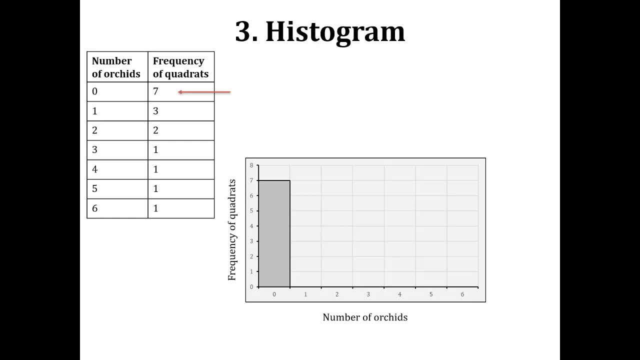 So we have our first block, which is zero number of arcades and the frequency of quadrates is seven, right. So this block represents our first observation, which is zero number of arcades in seven quadrates. Then we are going to take our second observation, and this observation is the. 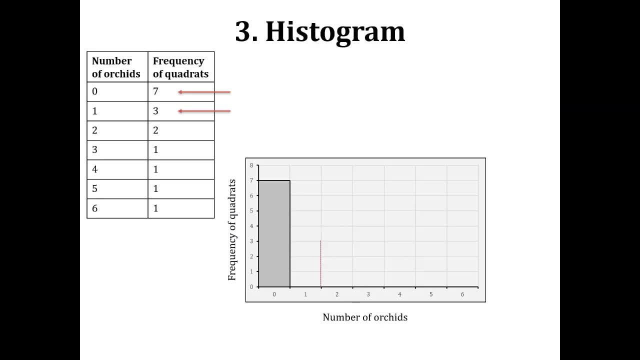 number of arcades one and the frequency of quadrates is three. So again we are with the help of the grid lines. we are going to locate that where our values are. So we are going to draw one line up to unit of one on the x-axis and we are going to draw a line from up to one on the x-axis. So here we have our next block. 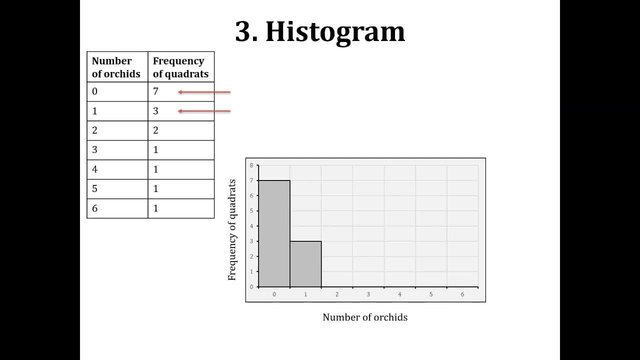 which represents the number of arcades and the frequency of quadrates in our second observation, And this is one and three, which means there are three quadrates which have only one arcade in them, And then we are going to draw the next blocks as 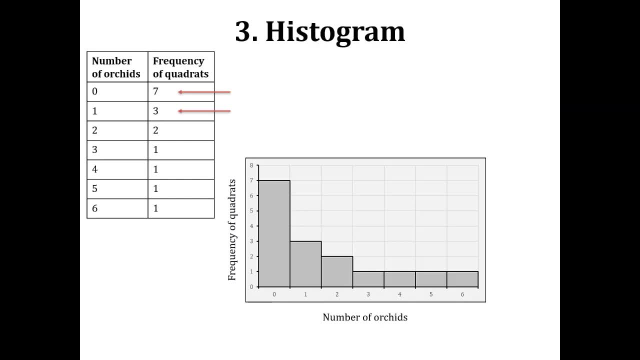 well. So this is how we make the histogram and the histogram blocks. you can see that these blocks, they represent the values on the x-axis and on the y-axis. So the first block represents the value on the x-axis as zero and on the y-axis as seven. The second block represents the value of one on. 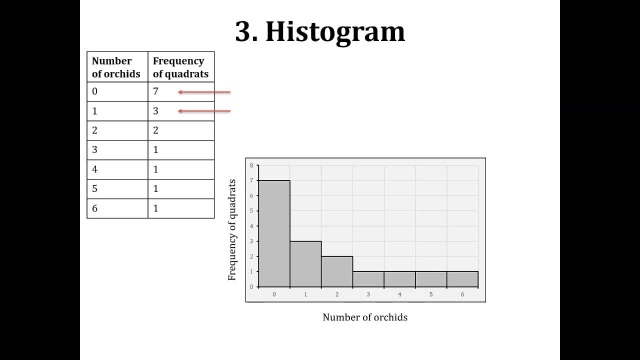 the x-axis and three on the y-axis. Then we have the third block, which represents the value of two at the x-axis and 2 on the y-axis, And then we have the blocks, the next four blocks that represent the value of 3,. 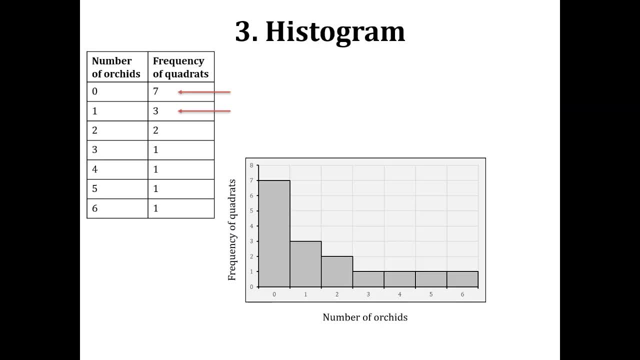 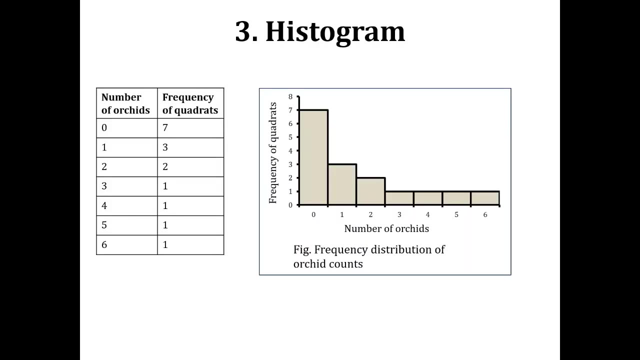 4,, 5, and 6 respectively on the x-axis and the value of 1 on the y-axis, right. So this is how we are going to make the histogram for the count data And, by removing the grid lines, you can have. 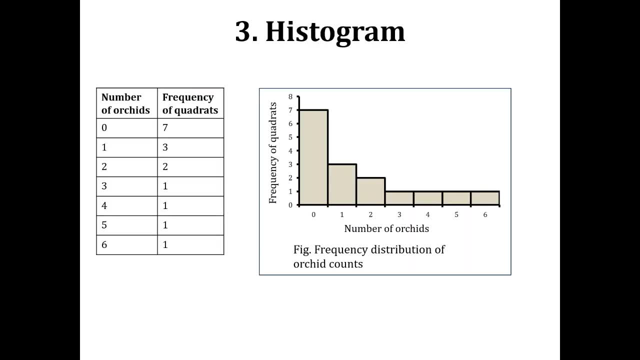 your final histogram And in the histogram, again, this has to be labeled And you can see that we have labeled the x-axis and we have labeled the y-axis, And also we have given the caption, which is the frequency distribution of orchid counts And again, just like the frequency tables, 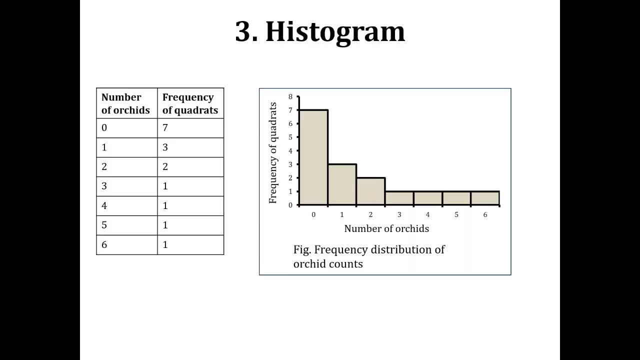 their labeling and their caption is particularly important that unless and until you have described the x-axis and the y-axis, and unless and until you have described that what this chart is about, you're not going to get the full credit. so this is the histogram of account data. now we are going to take the example of a. 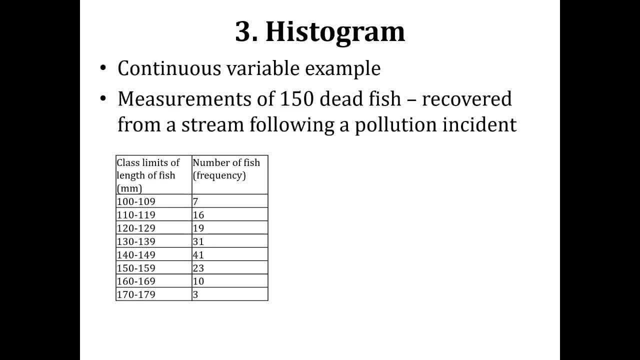 continuous variable, and this continuous variable is about the measurement of 150 dead fish and what this measurement is about. this is measurement about the total length of these dead fish that are recovered from a stream following a pollution incident. right, so here you have the frequency table, you have the 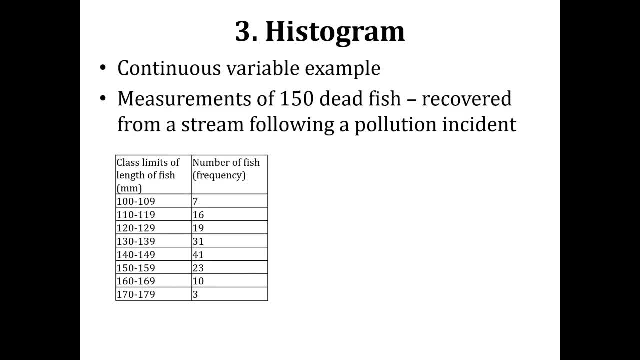 class limits of the length of fish and you have the number of fish which represents their frequency. so in the first class you can see that the observations they fall from 100 to 109 millimeters of length and the number of fish that fall into this class are 7. then we have the next class, which is 110. 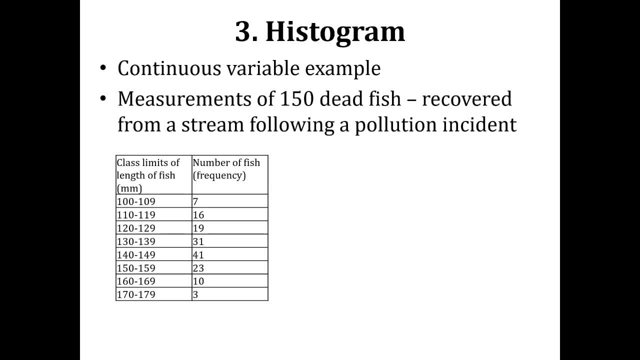 millimeters to 119 millimeters and we can see that there are 16 fish that fall into this class. now we are going to see that, how we can make the histogram for the this kind of the data. so here you have the histogram for this data and in this histogram you can see that we have made 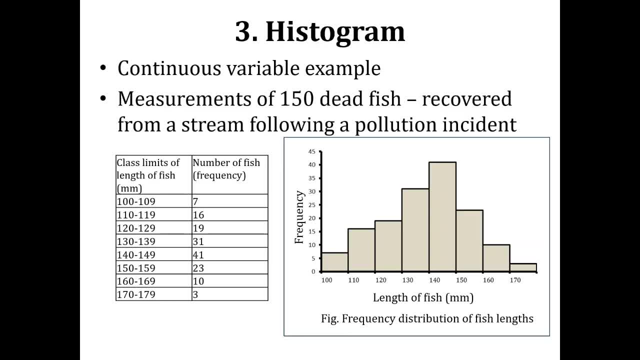 the blocks and how we have made the blocks: by scaling the length of fish on the x-axis and by scaling the frequency of fish along the y-axis. so we start our scale from 100 because our observation start from 100. so we are just simply starting from hundred and then the, the first block. 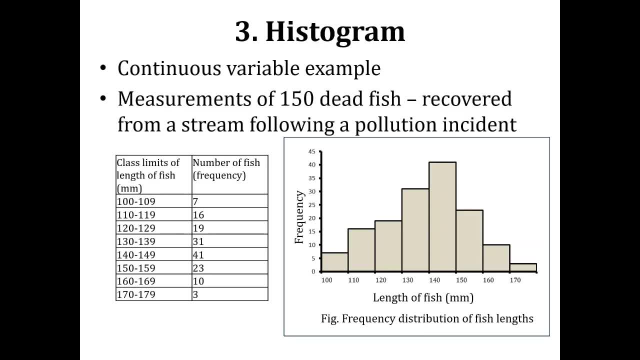 right, so the first block represents our first observation, which corresponds to hundred to 109 and the value of 7 on the y-axis. now, here you can see that we have the, which is continuous, right? So our first block starts from 100, and our next block is continuous. 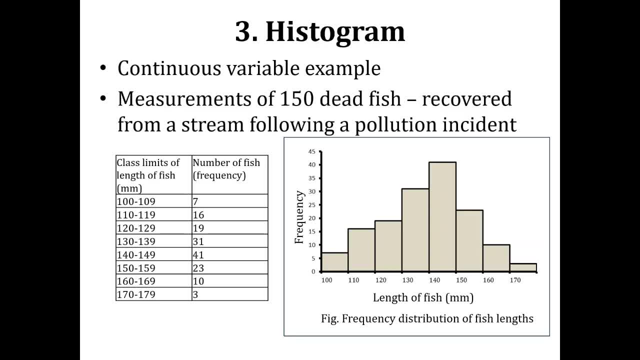 to it and it starts from 110.. Then our third block is also continuous and it starts from 120, which is the lower limit of the third class. So these blocks, why we said that these blocks or histograms? they are particularly useful for the measurement variable, because here you can see: 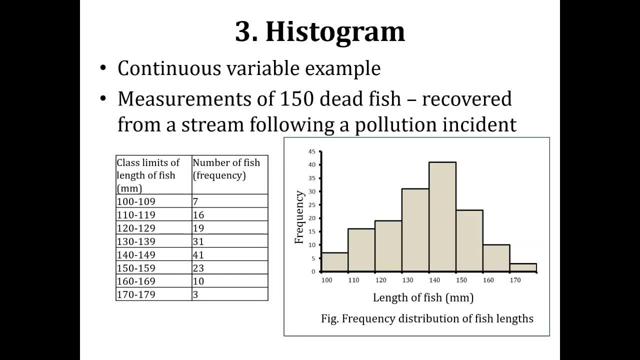 that we have a continuity of observations. So our first block starts from 100, and our next block starts from 110.. So our measurements are going to be continuous. So our first block is from 100 to 109, and our second block starts from 110, and it goes up to 119. Then our third block starts from. 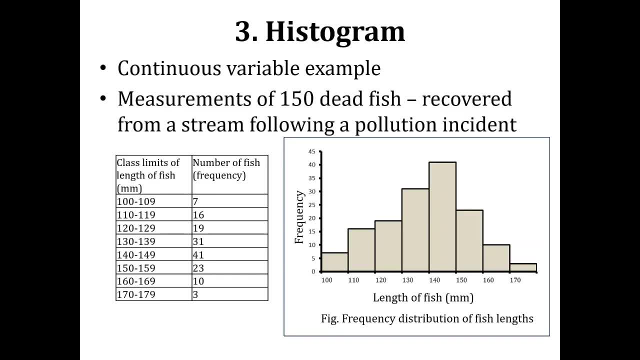 120, and it goes up to 129.. So here we have a continuous spread of the observations and these blocks. they represent the measurement data And again in this graph you can see that the data has become more visual, it has become more representative, and you can 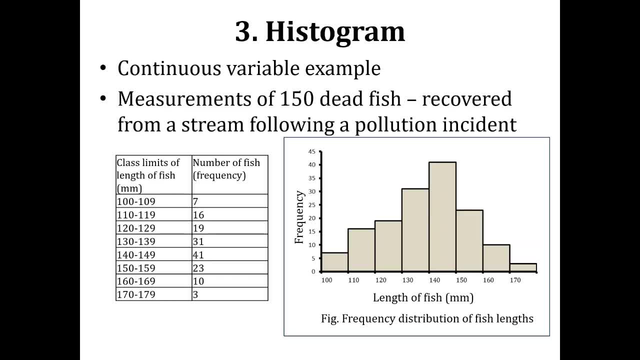 quickly see that. what are the trends in this data? that where the values are centered. So you can see that the values are centered in the middle right, So middle observations, they have most of the frequencies. So our observations are centered in the middle right, So middle observations they have. 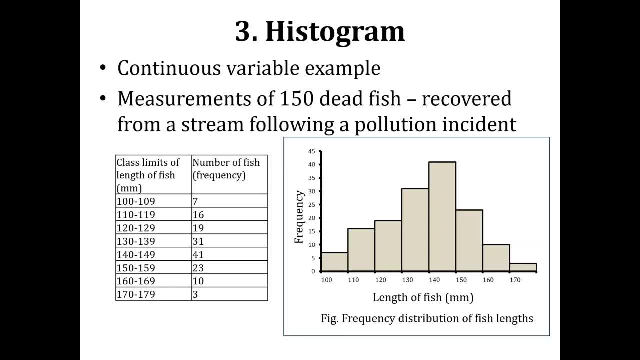 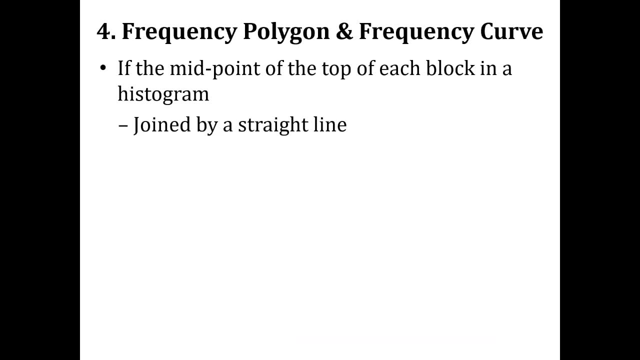 most of the frequencies. So middle observations, they are centered into the middle of this whole range of scores or all of these observations. So this is the histogram for a measurement data. Now we see the concept of frequency polygon and frequency curve And we can make a frequency. 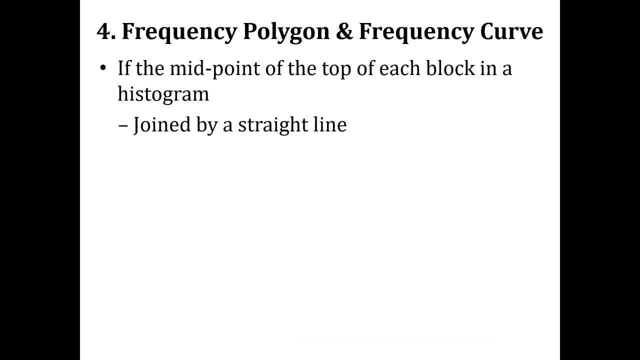 polygon or a frequency curve onto the histogram. And how we can do that is, the midpoint of the top of each block in a histogram is joined by a straight line, Then we are going to have a frequency polygon, Like in the example that we just saw, that we have the length of fish and their. 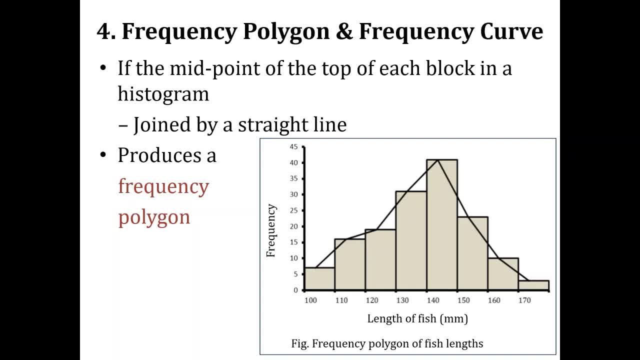 frequency is drawn on the y-axis. So if we join the midlines of these blocks then we are going to have a straight line And this line represents trends in their frequency. So it makes the data more representative And you can see that this is a frequency polygon. So when we draw this kind of 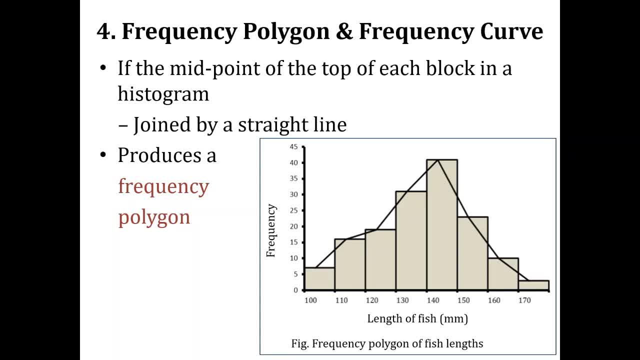 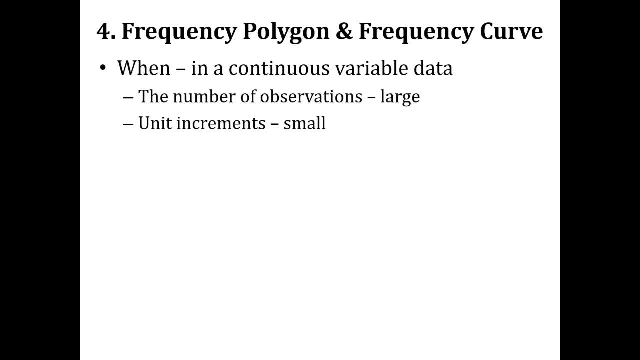 graph onto our histogram to show the trends more explicitly. then it is known as a frequency polygon. And when we have a continuous variable in which the number of observations are large and the unit increments or the unit steps are small, then usually we are going to have a smooth curve. So our 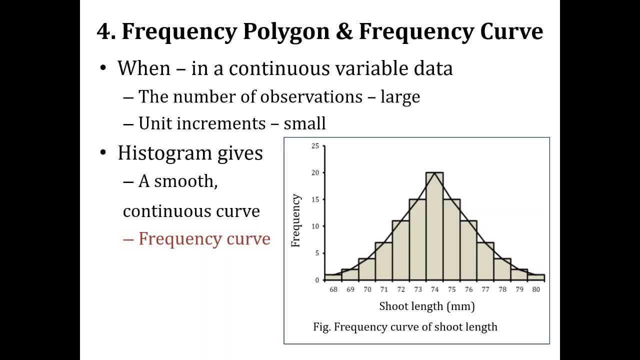 frequency polygon is going to be a smooth curve and this is known as a frequency curve. So this is a concept of frequency polygon and frequency curve. so here you have the example of short length, as we used in the previous lecture as well, that we were using this example to draw the frequency tables. so here we have the 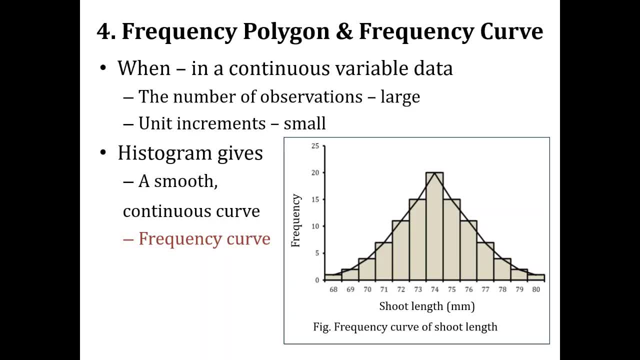 same observations and these are hundred observations and they fall in a spread or in a range of 13, right? so the unit increments they are 13, so they are small and the number of observations are large. so here, if we make the histogram and if we join the midlines of the histogram, this is going to give us the 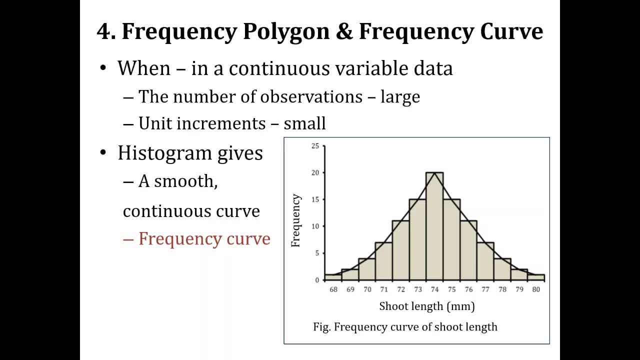 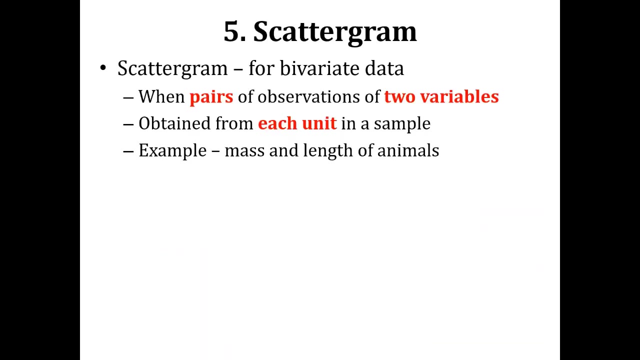 frequency polygon. but this frequency polygon is perfectly smooth, so this kind of the frequency polygon is usually referred to as a frequency curve. so this is the concept of frequency polygon and frequency curve: it becomes, it makes your figures or it makes your histograms more representative. now we see our next type of the graph, which is: 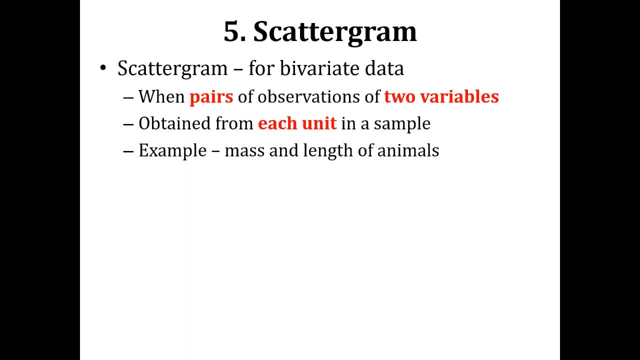 a scattergram, and scattergram is also one of the basic types of the graphs that are used in presenting the data, and the scattergram is particularly useful for representing the bivariate data. now, what is meant by the bivariate data? so by it means to, and variate relates to the term variable, so bivariate data is. 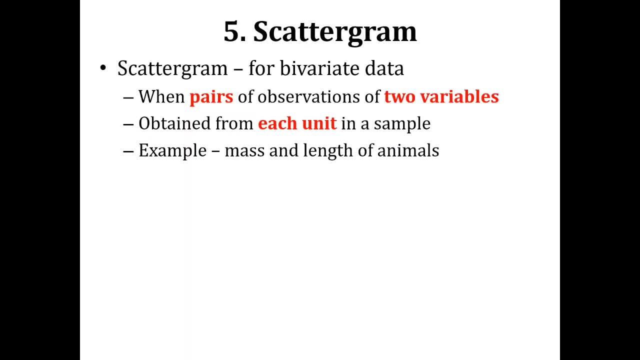 that type of the data when it's represented by the bivariate data. so it's just hanging and looking for some dynamics in your hieroglyphic yards, but that's why we use. but now we are going over to a Quando pathway path with our cameras and points looks like we. 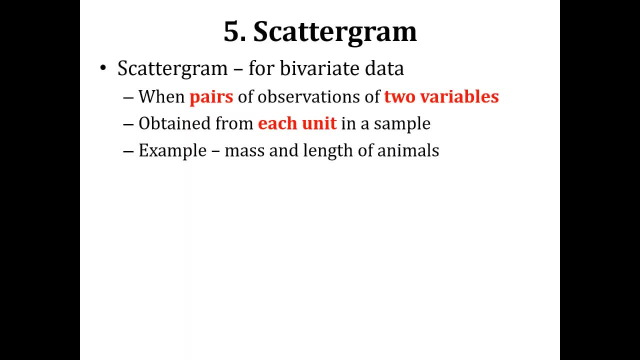 can have some numbers and it's asked, we can have any number of numbers in certain Sichuan- профессionalrays, as an example. I'm just checking out my computer right now and if I extend the data sosight and done a bit later, that's what that does. is that is the ž? give you these values and you do it, and that's. 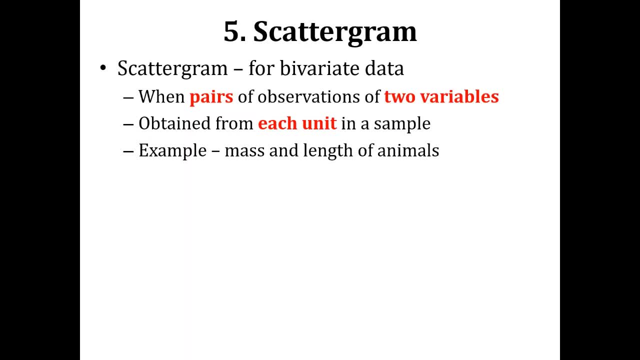 observations for two variables from the same sampling unit, from the same animal. so this is going to become our bivariate data, and it is why it is called bivariate, because we have taken two observations and these two observations are for two variables, two different variables, and therefore this is known as 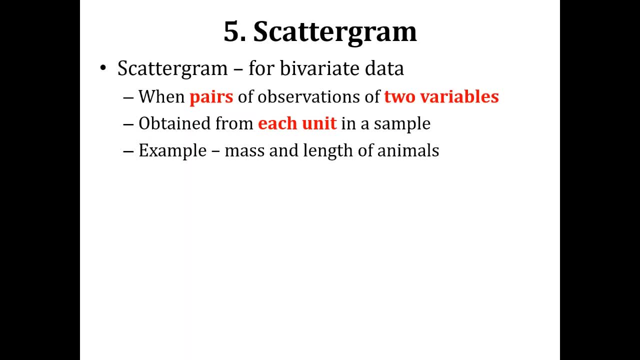 a bivariate data. now what we want to do is that we want to represent these two variables on the same plot. we want to represent these two variables on the same graph. so for that purpose, we are going to use the scattergram. we are going to make scattergram for this kind of a bivariate data and on the 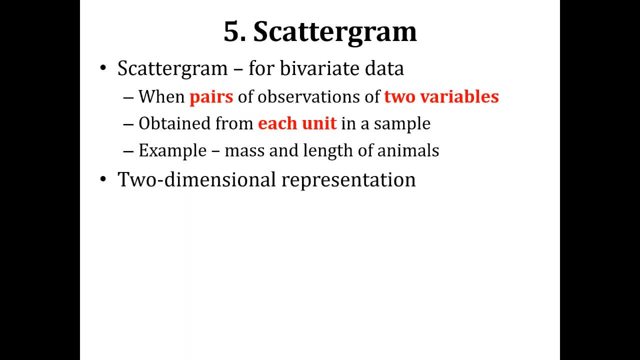 scanner gram. we have a two-dimensional representation. so two-dimensional representation means that we are going to present both of the variables and one of the variables will be taken along x-axis and the other variable is going to be taken along the y axis. so what variable should be plotted along the 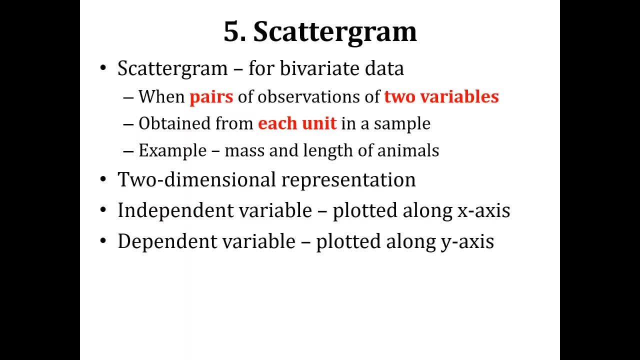 X axis and what variable should plot it along the y-axis? So it depends on the relationship between the variables, right? So if one of the variables is dependent on the other variable, then we are going to plot the independent variable along the x-axis and the dependent variable along the y-axis. For example, in case: 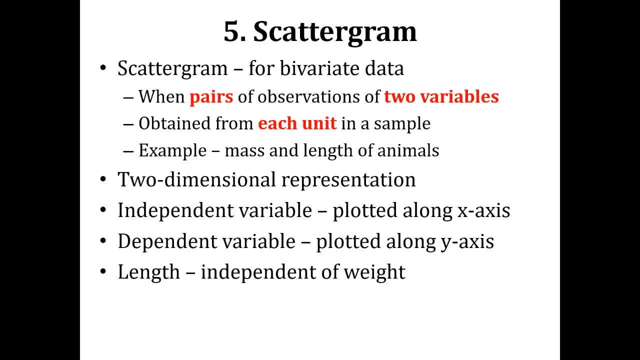 of mass and length. we can see that length is independent of weight, right? While weight is somehow dependent on the length of the animal. So the animal, as it becomes lengthier or it becomes taller, it is going to have more weight, right? So weight is somehow. 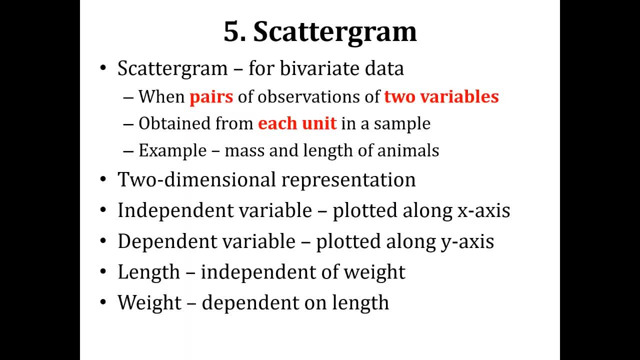 dependent on length when it comes to the relationship between these two variables, right? So weight is not just dependent on the length. There are other factors that contribute to the weight as well, to the weight. But when it comes to these two variables, and we want 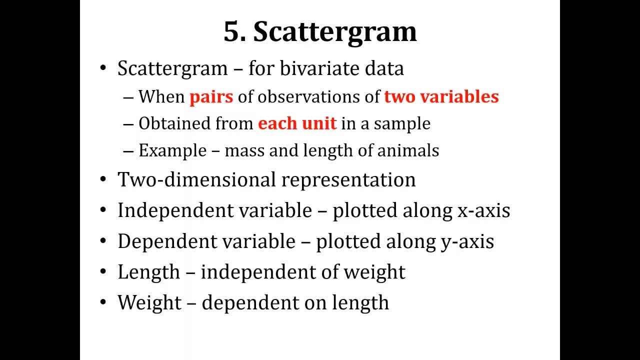 to see their relationship to each other. then we can see that length is something which is not dependent on the weight, while weight is dependent on length. So, in case of these types of variables, where we can define that which one of the variables is independent of the other and which, 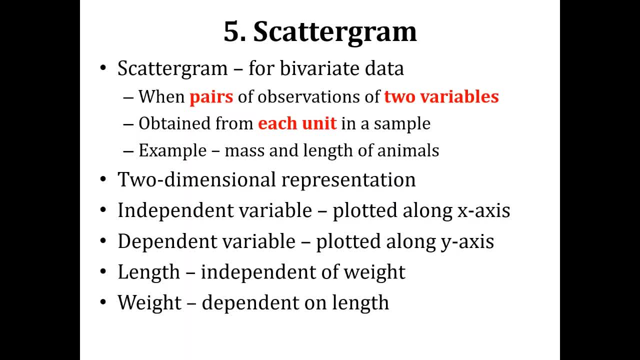 one of the variables is dependent on the other, then we are going to plot the independent variable along the x-axis and the dependent variable along the y-axis. But if we have the observations which are not related to each other and still we want to draw them on the scattergram. 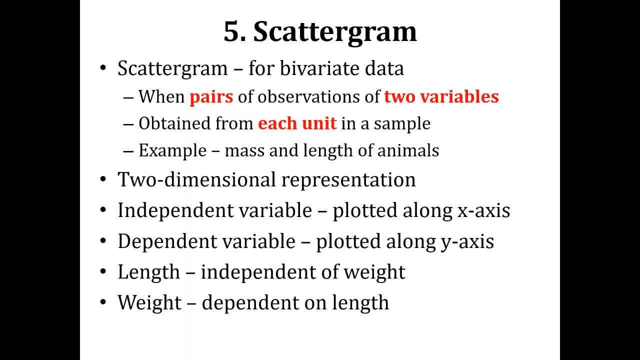 then we can plot any one of them along the x-axis and any one of them along the y-axis, right? For example, if you take the measurement of the serum glucose level from a patient and you also take the measurement for their blood pressure and you want to represent these two. 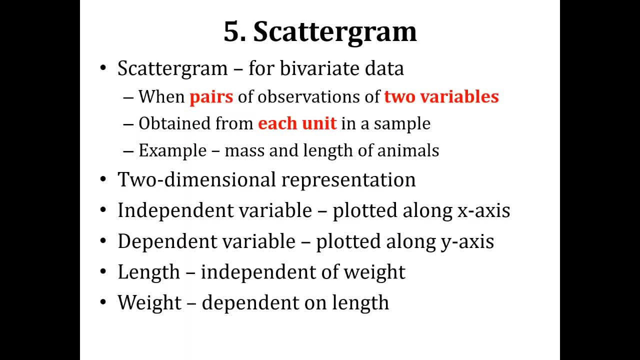 both of these variables on a single plot, then you're going to use the scattergram And in the scattergram you can plot any one of them along the x-axis and any one of them along the y-axis, because these two, they don't seem to have a relationship between each other, that which one is dependent. 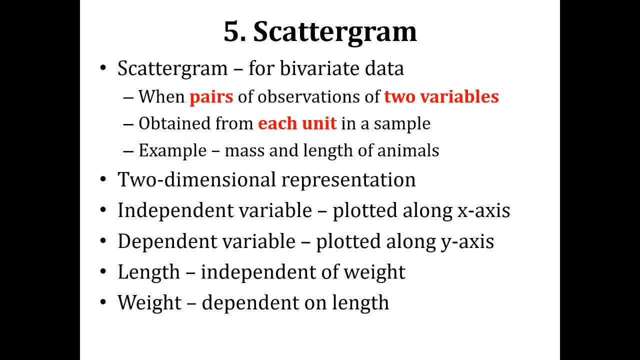 or which one is independent. right, But still, these scattergrams are used to find out the relationship, and we will. we will see how. right, But if you don't have pre-information that one variable is dependent on the other or the versa, then we can plot any of the variables along any of the axes. 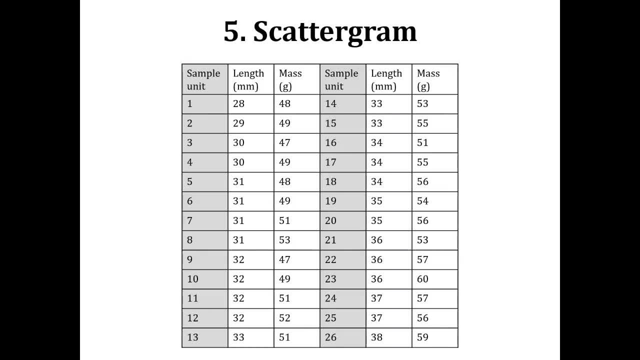 So here we are going to take the example of mass and length of the animals, and how many sample units do we have? We have 26 sample units and we have measured two observations from each of these 26 sampling units. And these two observations, they relate to two variables: One is length and the other 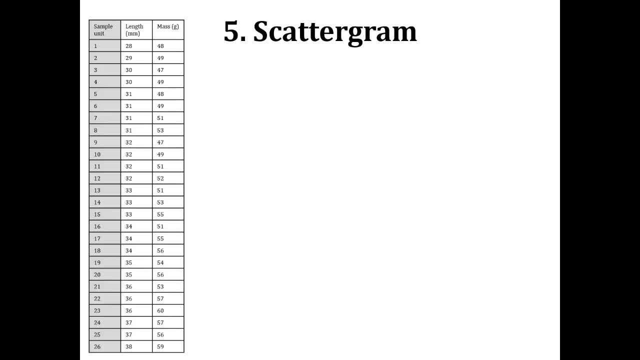 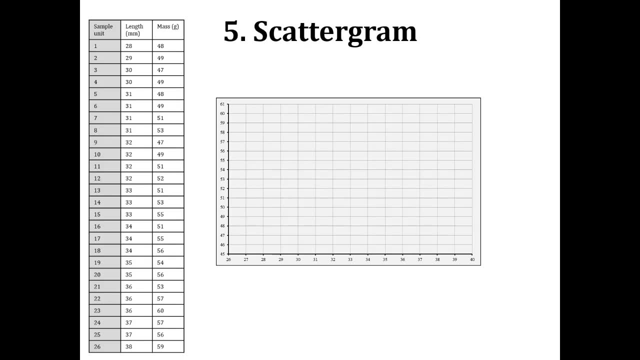 one is mass. Now we are going to make the scattergram for these two variables and here we have the basic outlay of our scattergram and you can see that we have x-axis and the y-axis and on the x-axis we have the length of the animal because, as we discussed that when it 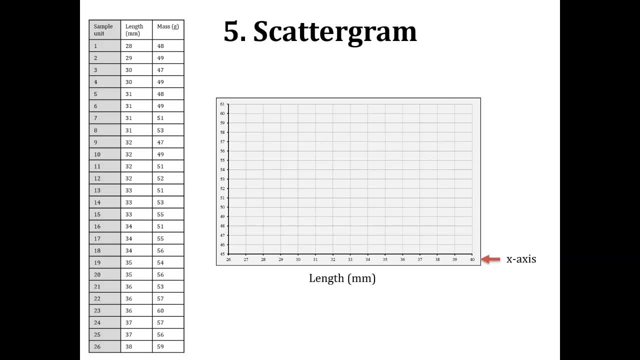 comes to the relationship between length and weight, length is independent of weight, while weight is slightly dependent on length. Therefore, we are going to take weight or mass along the y-axis. So here we have our axes defined And what we have is what we are going to convert into x or y. So it Summit metal. 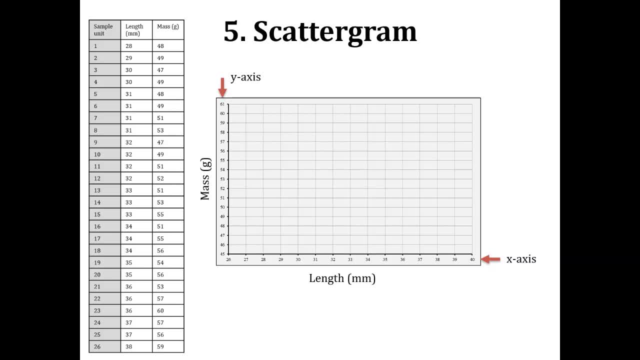 which one is x-axis and which one is y-axis. Now let's see the scale on these axes. So here we are not starting from 0, so we are starting from 26, because our lowest observation in length is 28. so we are starting from 26 and our lowest 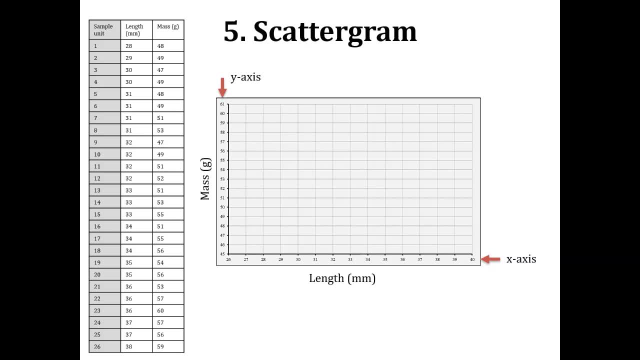 observation in the mass is 47, so we are going to start our graph from 45. so this is up to you, that from where you want to start your scale, because if you are going to start from 0, then it is going to become less informative, right, and we? 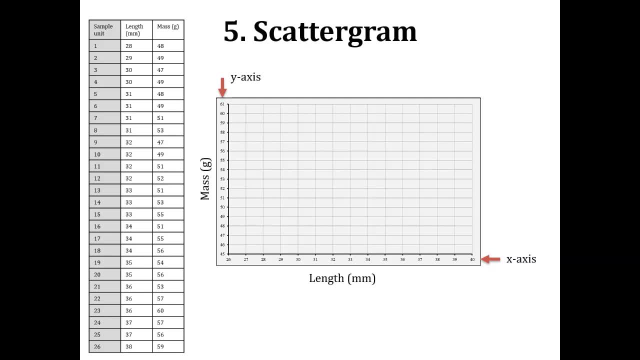 will see a comparison that if we start from 0, then what kind of a graph we are going to have, right? so for now we start from 26 and 45. so we have the grid lines here and we have the y-axis grid lines. we have the x-axis grid lines. 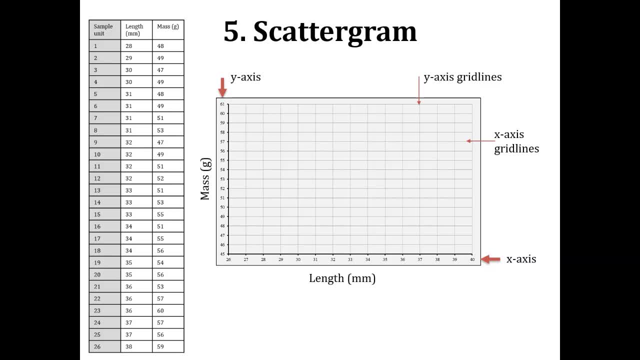 and we have the y-axis grid lines and what these grid lines are for. so these grid lines, as we discussed earlier, that these grid lines, they are going to help us in making the scattergram when we are going to make it on paper. we are going to make that manually because it will, these grid lines, they will enable. 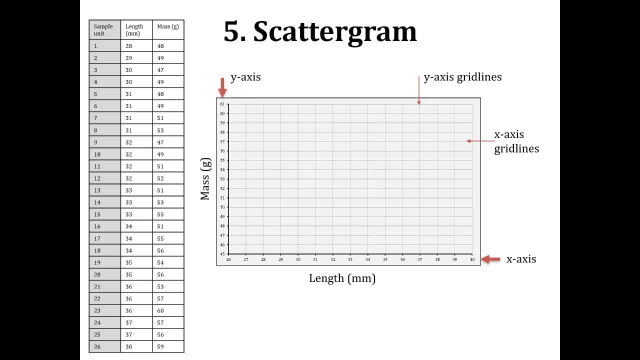 us to scale our observations on to the chart area, right? so, starting from the first observation we have, we have 28 and 48, so it means that this is going to the place where we are going to mark our observations, and this place is 28 along the x-axis and 48 along the y-axis. so we are going to 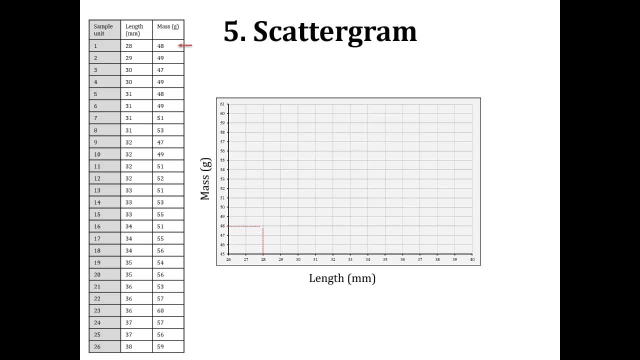 point out a point on the chart, area which corresponds to the x-axis value and its y-axis value. so here we have pointed out that area and we are going to place a dot over here, right, so we are going to place a marker over here which is going to represent our bivariate observation and 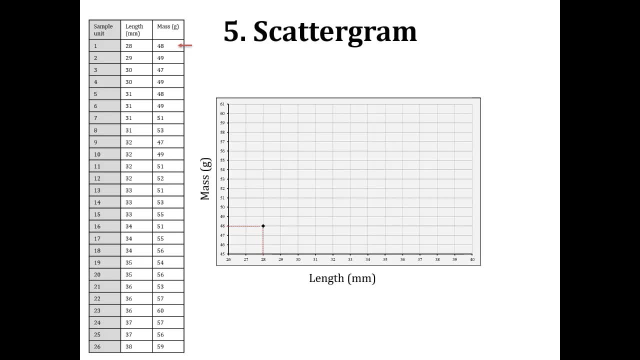 this mark. it relates to 28 value on the x-axis and it relates to 48 value along the y-axis. so here we have placed our first observation in the form of a marker. then we have our next observation, which corresponds to 29 and 49. so again, 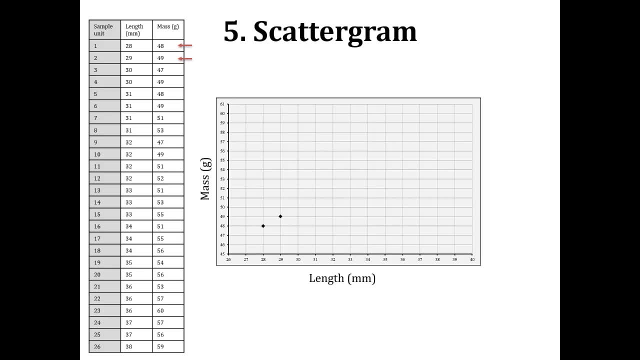 we are going to mark out the area and we are going to place a marker or a dot on that area. and we are going to mark a dot or a dot on a star or a diamond or on any kind of a marker. you can have a star, you can have a circle, you can have a diamond. 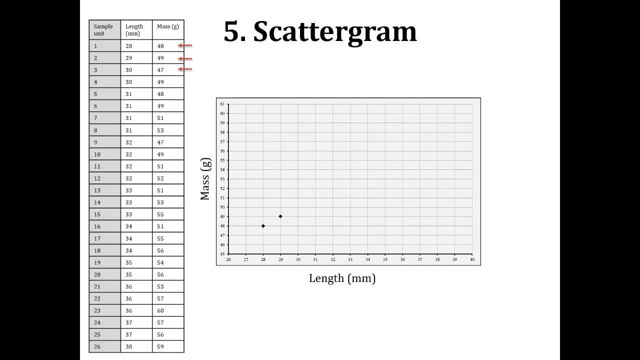 shaped marker, so you can have any type of a marker, and then you're going to mark all of the observations in your chart. the next observation is 30 and 47 and you can see we have the this marker. this marker represents 30 along the x-axis. 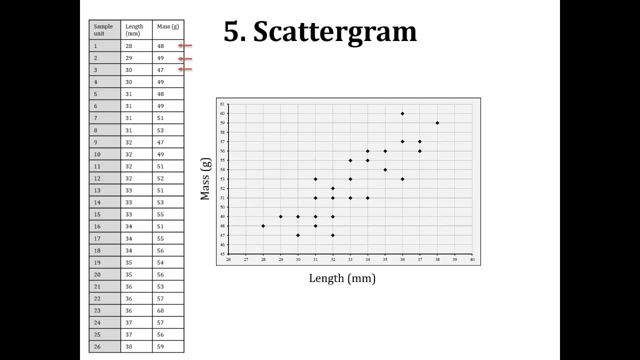 and this marker represents 40 along the y-axis. and again we are going to place a dot over here, going to have all of the observations marked on our scattergram. So why this is known as the scattergram? Because it shows the scatter of the observations of two variables in a single graph. 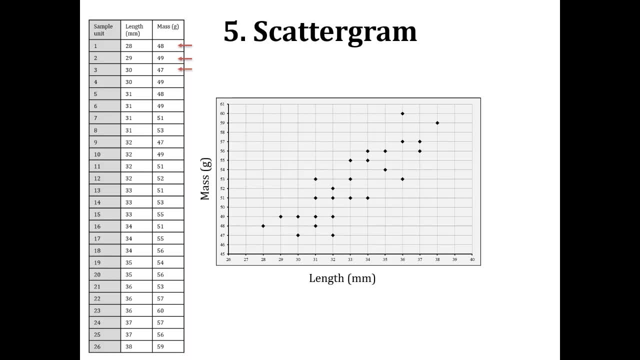 So this is a two-dimensional representation, right? So why two-dimensional? Because each marker right, each marker on the chart- it is representing two variables at a time, right? So each marker is representing two variables. So therefore, this is known as a two-dimensional representation. 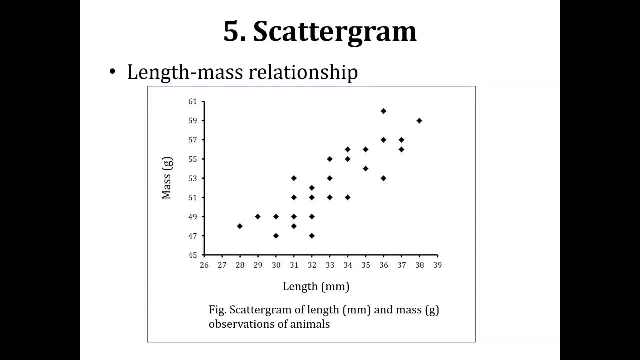 Now, after removing the grid lines and removing the chart background color, we are going to have our final figure in this form. So this is the scattergram, And this scattergram is about the two variables, which are length and mass, And you can see that we have properly labeled. 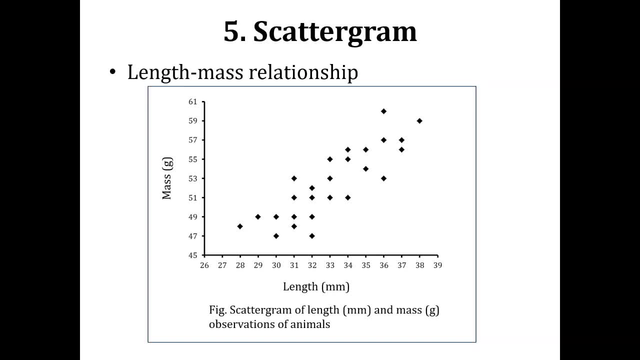 these variables, The length is along x-axis and the mass is along y-axis, And we also have given the title or the caption of this figure, which is the scattergram of length and mass observations of animals, And you can see the scatter or the spread of the observations. 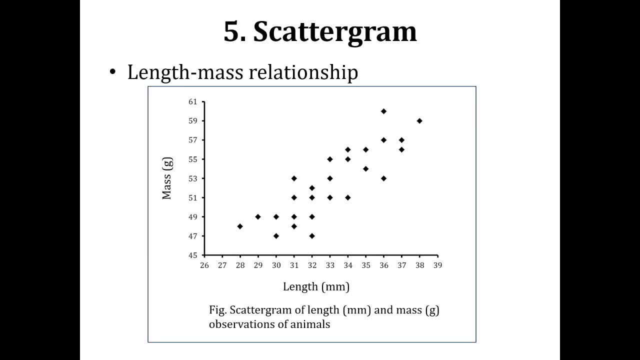 over here. So this is the scattergram that we have Now. this scattergram is about the relationship between length and mass And we can see that, how we can describe this relationship, that what is the purpose of making this scattergram, And here you can clearly see. 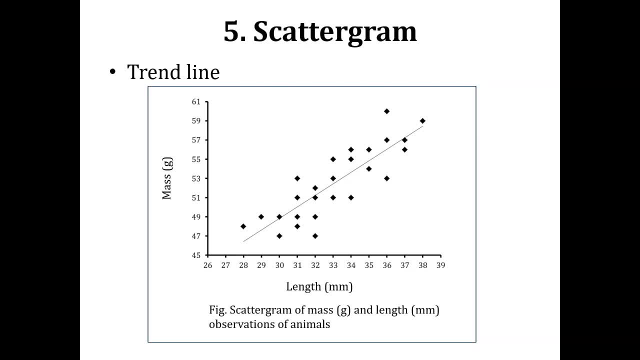 that if we draw a straight line across the scatter of these observations, which is known as the trend line, we can see the trend. And here we can see that, what is meant by the relationship between two variables, that what is the purpose of drawing these two variables together, As we discussed. 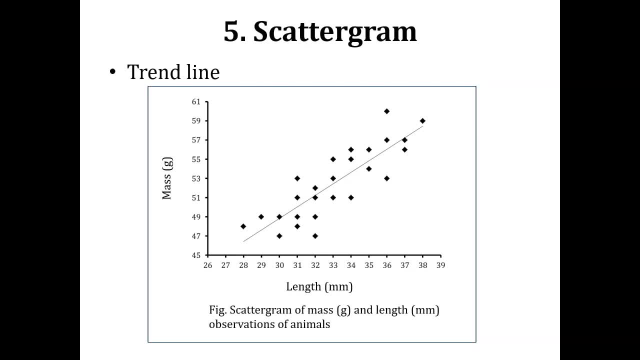 that scattergram is the two-dimensional representation, that it represents two variables at a time. So we have two variables- length and mass- And why we are plotting them and why we are making a scattergram, why we are making a two-dimensional picture, is because 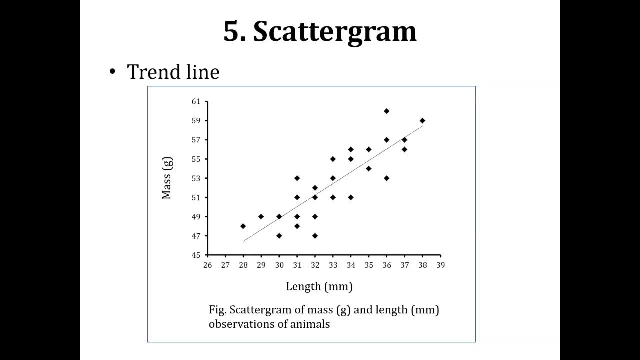 we want to see the relationship between them, And this relationship can be seen by making the trend line, And here you can see that we have a positive trend line. We have a positive straight trend line here, which means that with increasing length we have increase in. 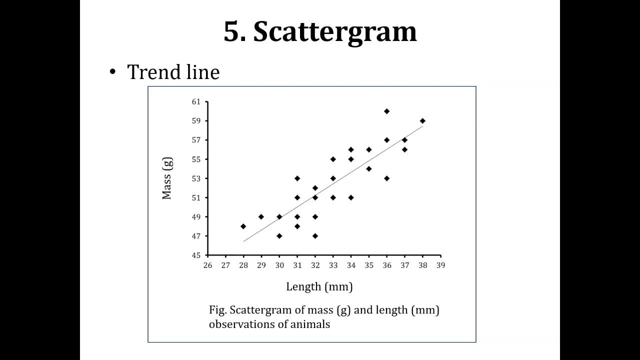 mass as well. So this is how you can see the relationship between these two variables, that we can see a common trend: that as the length of the animal is increasing, the mass of animal is also increasing. So this is what is meant by a scattergram and why this scattergram is used. 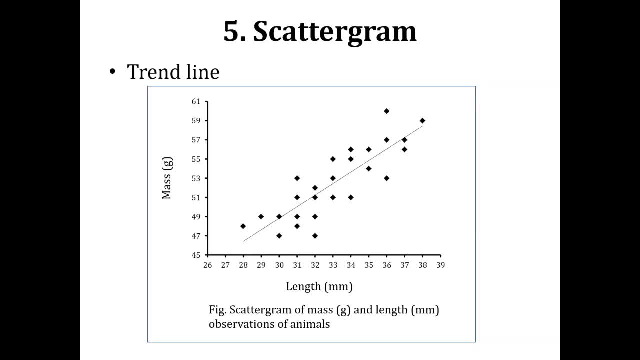 So scattergram is used to represent two variables by the read data, when two variables are taken from each sampling unit in the population, And what kind of the scatter or what kind of representation this one is. So this is a two-dimensional representation in which we are 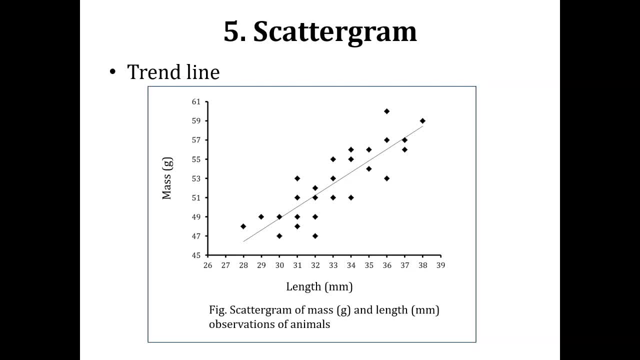 representing two variables right. And why this is known as two-dimensional? Because we are presenting two variables and each marker on the plot right, each dot or each marker on the plot that belongs to two variables, that represents two observations at a time. That is why this is. 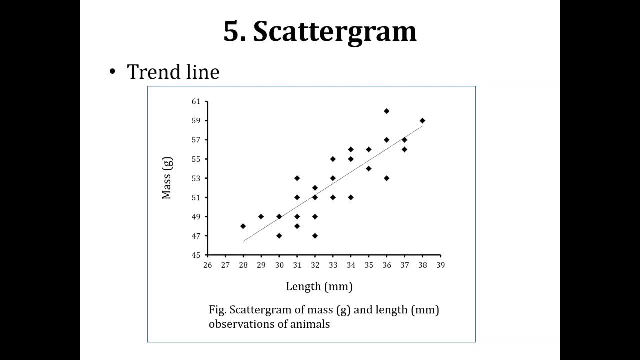 two-dimensional right. And the other thing that the why we use the scattergrams is that because we are plotting the two variables and we want to see their relationship right. So because it is two variables, therefore, we are going to make the scattergram. So this is the purpose of making. 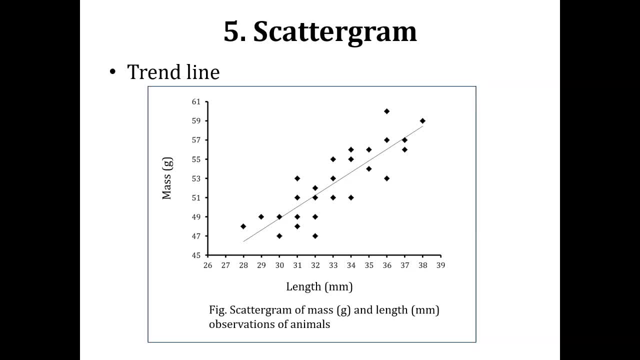 scattergram that we have two variables and we want to see the trends, that if we increase one variable, that if we increase the variable which is plotted along the x-axis, then we can see that what is the effect on the variable on the y-axis. And here you can see that the observations are. 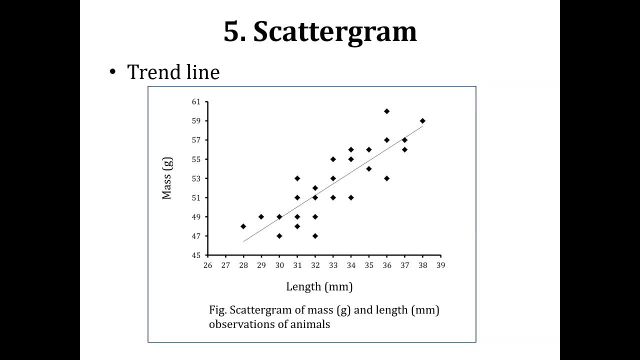 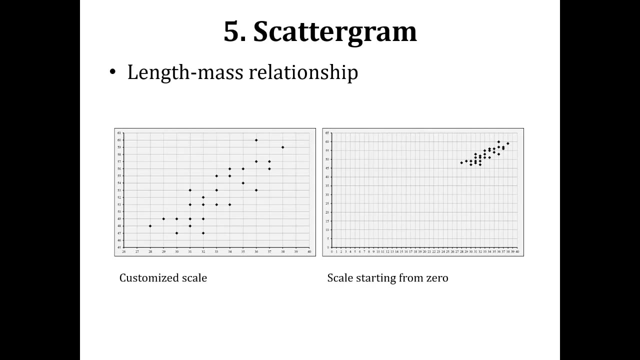 scattered in such a way that as we increase the length of the variable, we can see that the length we are also seeing an increase in the mass. So this is what scattergrams are used for, And here we can quickly see the choice of our scales, the choice of the units on our scale. 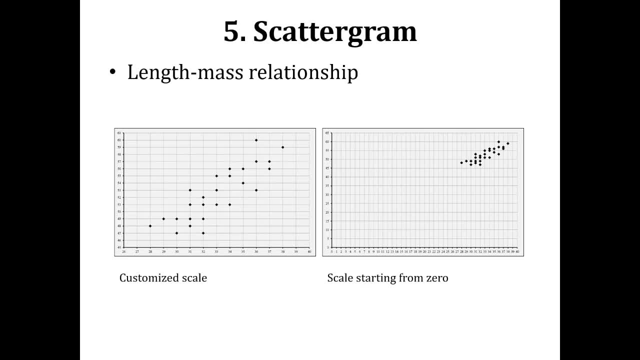 that from where we want to start our scale, And here you can see that we have the scale that starts from 26 and 45, our customized values, And here is the scale that starts from zero. So you can clearly see the difference in their presentation. 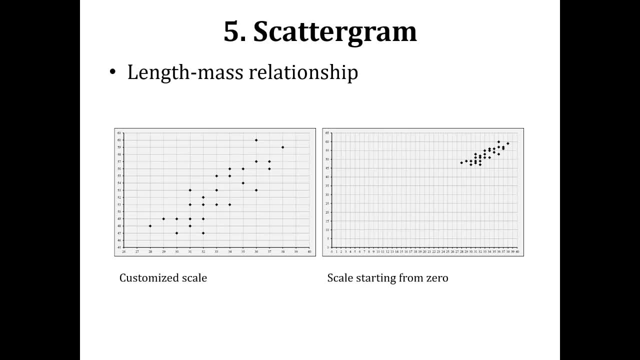 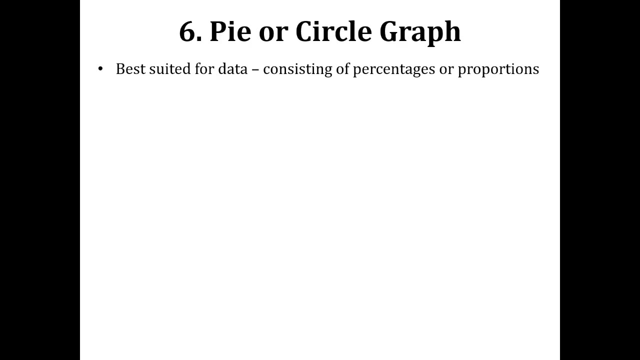 That which one of these figures is more informative and which one is less informative. So this is the purpose of customizing your starting points on the scale that you want to make your data more representative. Now we are going to discuss the pie or circle graph. 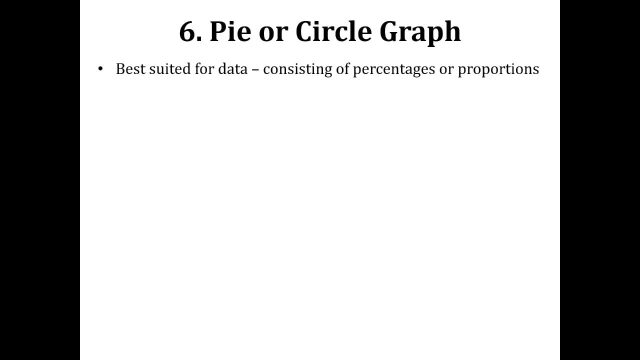 And the pie or circle graph is also one of the basic types of the graphs that are mostly used in biological research, And this type of the graph is suitable for the data which consists of percentages or proportions of different activities or different categories, And we are going to take the example of. we are going to actually take two examples. 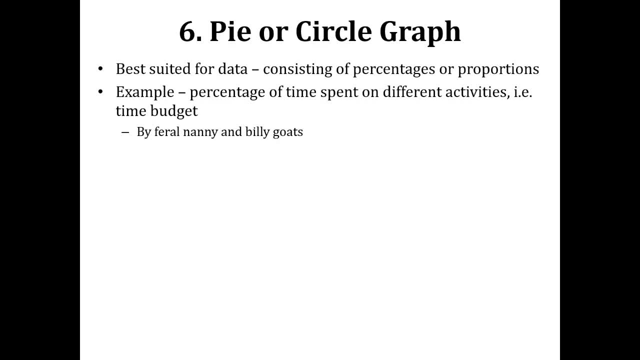 And these examples are from the goats species, the nannies and billies- the nanny goats and the billy goats. And what is documented in this example is that their percentage of time spent on different activities, which means that it is their time budget analysis: The percentage. 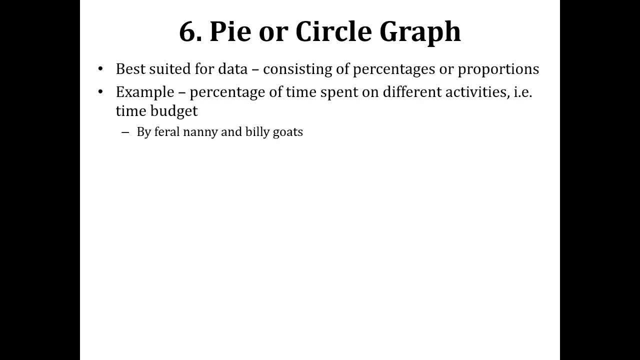 of their time in a day that they spent on different activities, right? So this is the observation that we have, And here in the table you can see that their activities have been mentioned. Different categories of their activities have been mentioned. They are feeding, lying, standing. 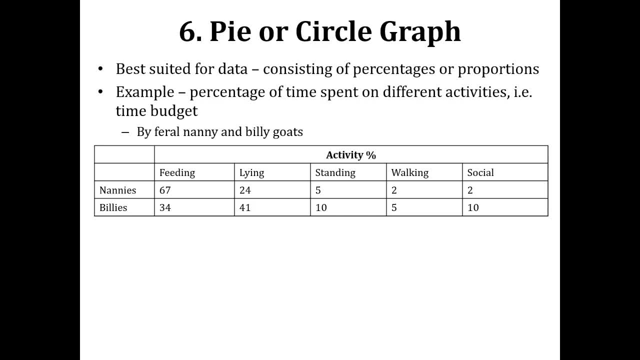 walking and their social activities, And the percentage of time which is spent in each of these activities is also shown against both of the species. So we have nannies which spend their 67% of the time in feeding, and we have billies which spend their 34% of the. 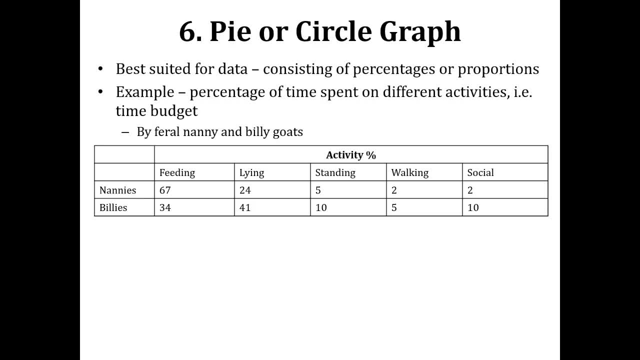 time in feeding And we can have the. we can see the percentages of all these activities by the two goat species. Now we want to see in the form of the graph, that which activity takes most of their time. So here we have the activity budget graph for nannies And. 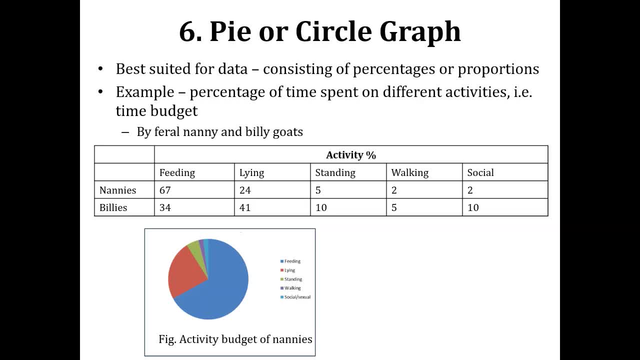 in this you can see that the different activities have been presented. They are represented by different colors, Like the feeding is presented by the blue color, lying is presented by the red shade, The standing is presented by a green shade, Walking is presented by a purple shade and social is represented by a zero shade right. 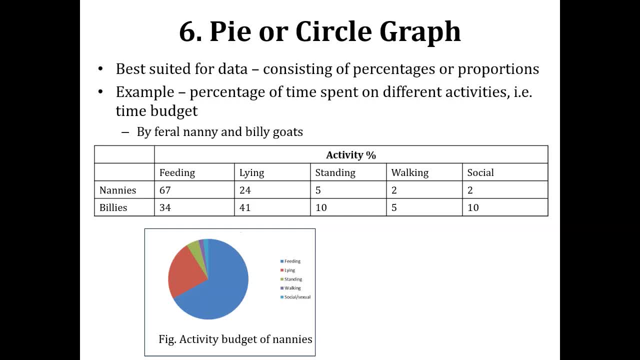 So we have different colors and shades that represent different activities, And in this figure you can quickly see that most of their time is spent in feeding. right, So they spend most of their time in feeding And they also spend most a major proportion of their time lying And they spend least. 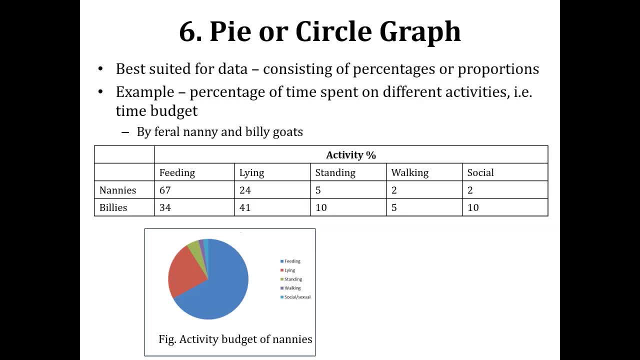 of their time in walking and in social activities. So here you can quickly see the percentage of time spent in different activities. And now you can compare that with the table that- although in the table you also have mentioned their values, their percentage time spent.